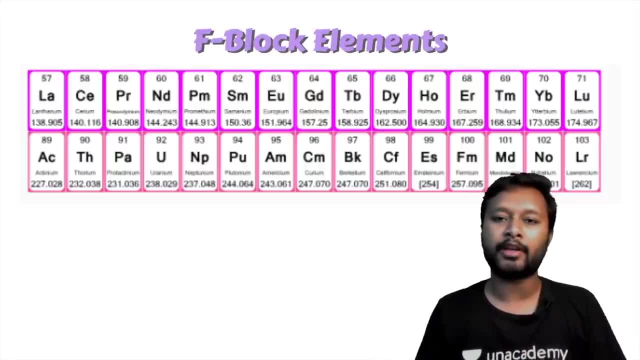 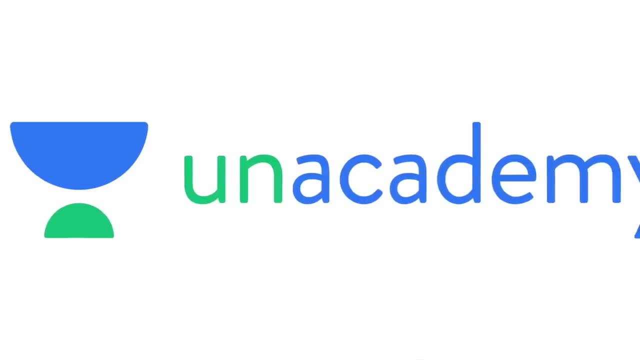 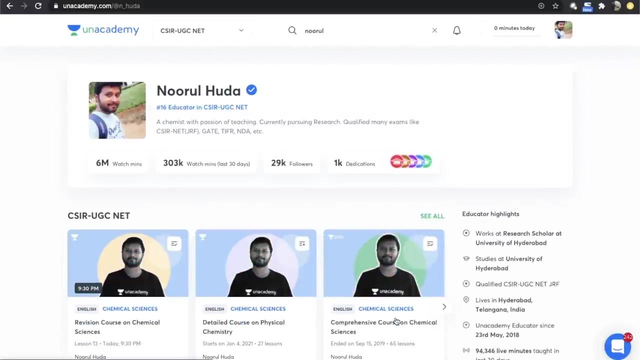 It won't be containing each and everything from the F block elements, but yet it will contain the most important things which you need and with which, with the help of which, you will be able to solve questions in the exam. So that is something which you are going to get in this particular video. Now, before starting this video, before going into that, let me tell you that I teach on an academy platform and the courses are running over there on an academy plus regarding the revision of CSI net exams. If you are interested in that, you can join an academy and you can take the subscription of that. 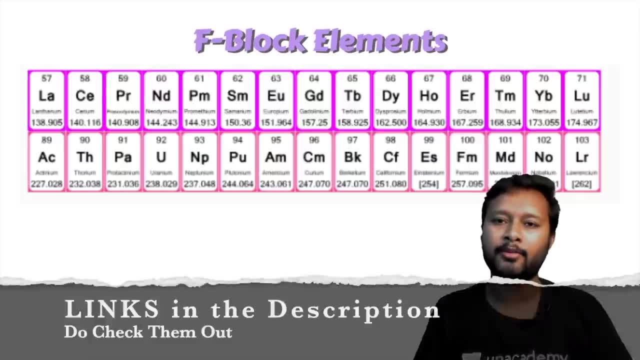 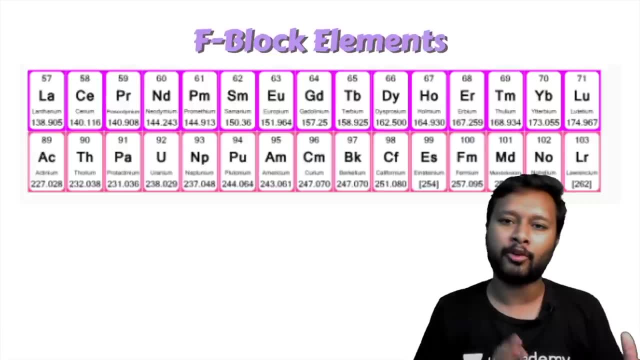 Do visit my profile on an academy. There are videos on F block elements where I have explained whole concept and also discussed about the questions over there. The link for the for my profile of an academy is there in the description of this video, So do check that out right Now. coming back to the video, So here I'm going to just talk about lanthanides and actinides. What are the important terms in this, What are the things which you need to know? And at the end of this video I'll tell you some of the important terms which are there associated with this. 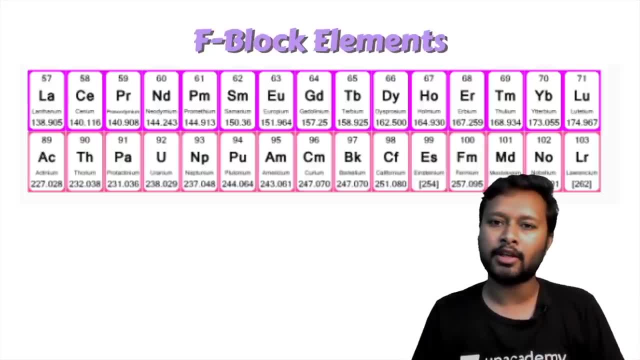 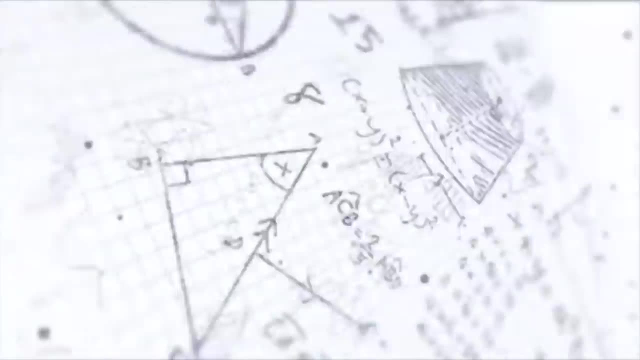 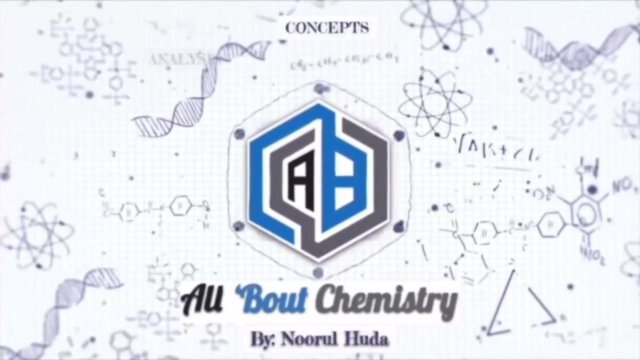 Particular F block element whose definition and whose explanation is needed. Okay, So that's how this video will be done, So let's straight away get into the video. All right, So the first thing which we are going to do is we are going to talk about the 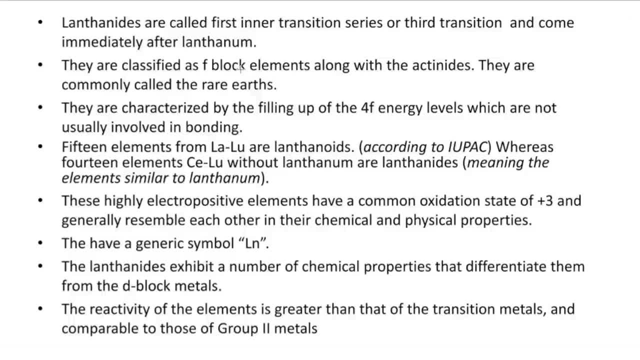 lanthanides and actinides is their common properties, like their introduction kind of thing. That's what we are going to do. So, first of all, these lanthanides are called your first inner transition series, or the third transition series, That's what you can call them, And they come immediately after lanthanum, which is a D block element. Right Now they are classified as F block elements, along with the actinides. They are commonly known as rare earth metals, So that's what is the name of them Like. that's what the name given to them is: a rare earth metals. 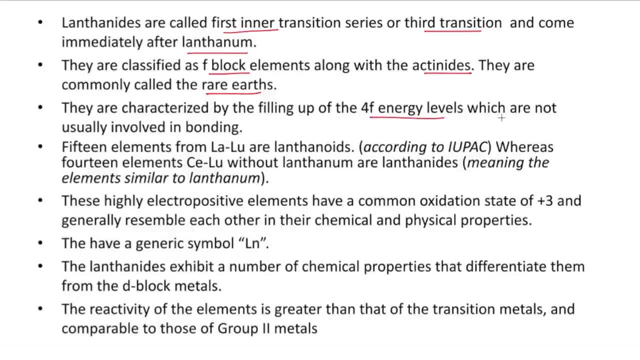 Now they are characterized by filling up of 4f energy levels, which we all know and which are not involved in bonding. So understand this: that these 4f orbitals are not involved in bonding. The next point is that 15 elements from lanthanum to lutetium- these are called as your lanthanoids. 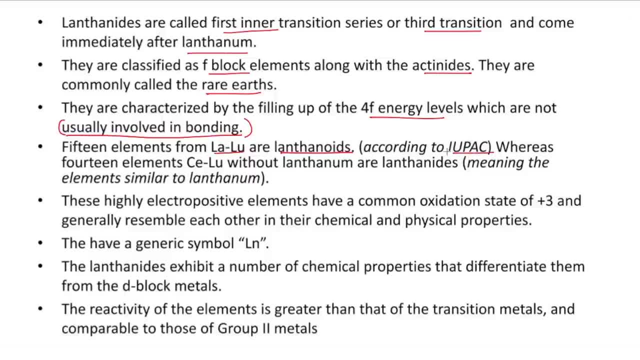 according to the IUPAC naming, or IUPAC naming, whereas the 14 elements starting from your cerium to lutetium without lanthanum. these are called as lanthanides. So understand the difference: lanthanoids and lanthanides when they are. whenever it is asked about lanthanoids, 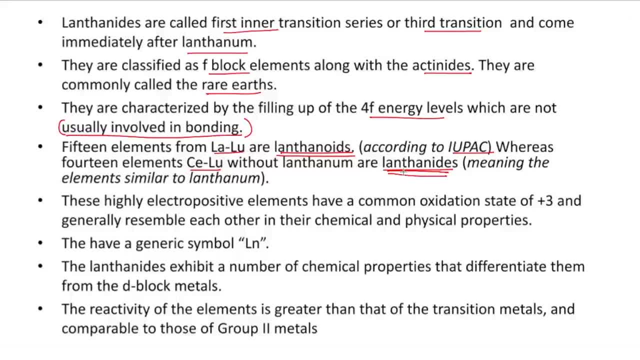 you have to consider this lanthanum, and when it is asked about lanthanides, you have to exclude lanthanum. you have to start from cerium, right? So that is what it is. that is according to the IUPAC naming. Now, these high, these are highly electropositive elements and they have common 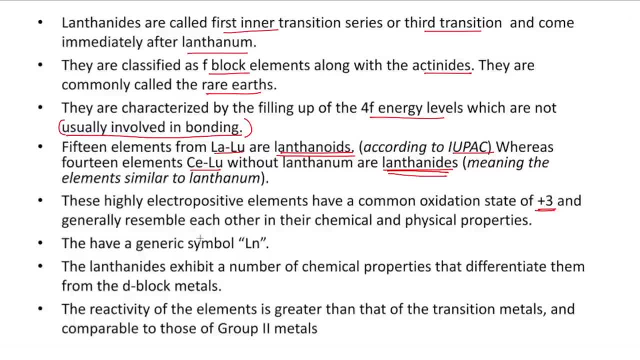 oxidation State of plus 3 and the general generally resemble each other in their chemical and physical properties. So the chemical and physical properties of all these lanthanides and actinides are quite similar to each other. The generic symbol which is given to them is ln, So whenever 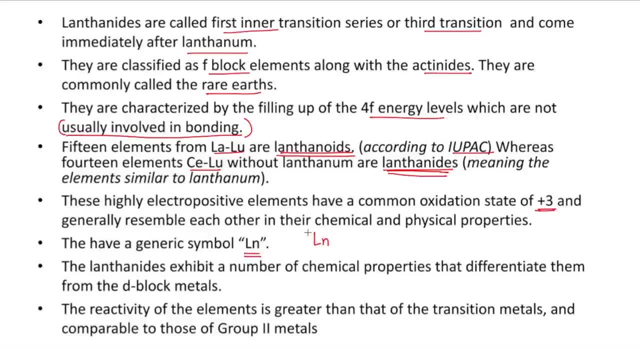 a ln is written, that means it is specified about all the or it is just a general symbol given for all the lanthanides. So if a certain property will be associated with all the lanthanides, it will be expressed in the form of ln. The lanthanides exhibit a number of 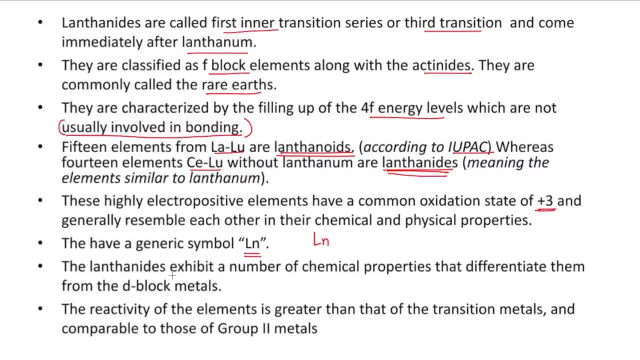 chemical properties that differentiate them from the d block elements that we will get to know in the further slides. The reactivity of the elements is greater than that of the transition metal and it is comparable to that of group 2 metal. So you should know. 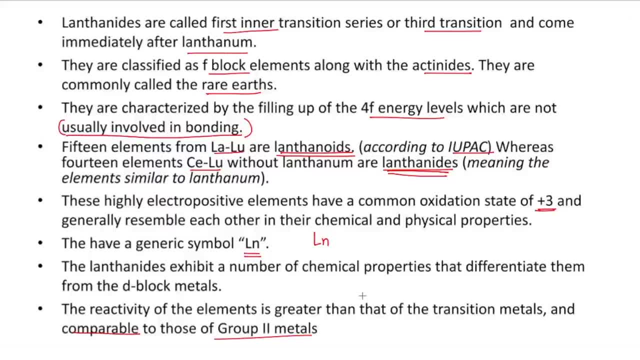 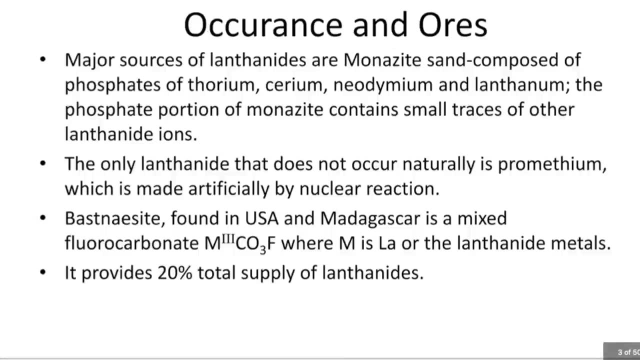 this thing, that these f block elements have similar or comparable properties to that of group 2 metals also, and they are quite more reactive than your transition metals. Let's talk about their occurrence and ore that in what are the ores and all? so the major source of lanthanides are your. 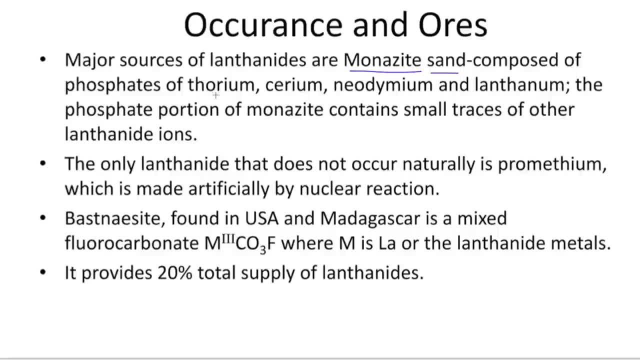 monazite sand and basically they are composed of your phosphates of thorium, cerium, neodym and lanthanum. right, the phosphate portion of monazite contains small traces of other lanthanidin as well, but that's not of the more importance. the more importance is that that monazite sand is actually 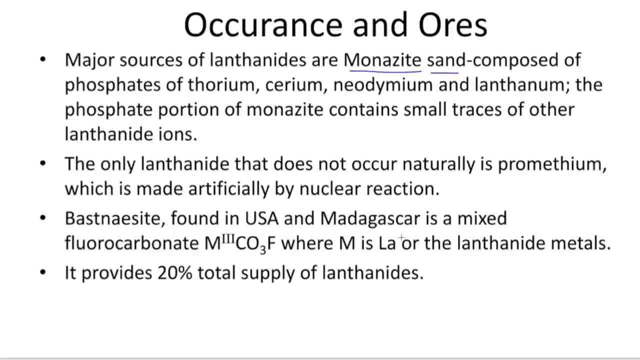 phosphate of thorium, cerium, neodym and lanthanum. the only lanthanide that does not occur naturally is promethium. now, this is a very, very important point. just mark this thing: that the lanthanide which does not occur naturally is your promethium, and this is made artificially by the nuclear. 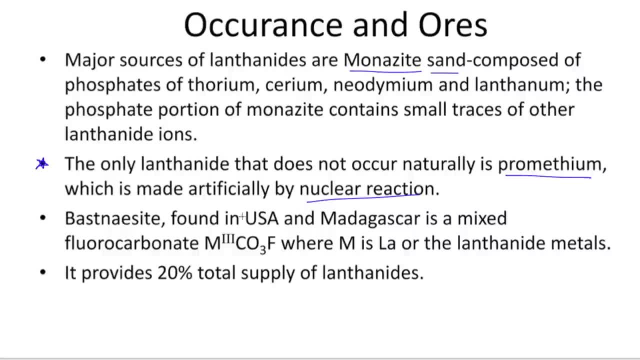 reactions okay. so this is a very important point. regarding your lanthanides and basnicite, which is found in usa and madagascar, is a mixed fluorocarbonate in which metal is in plus three oxidation state, co3f, where m is your lanthanum or the lanthanide metal. remember we are not talking about lanthanoid. 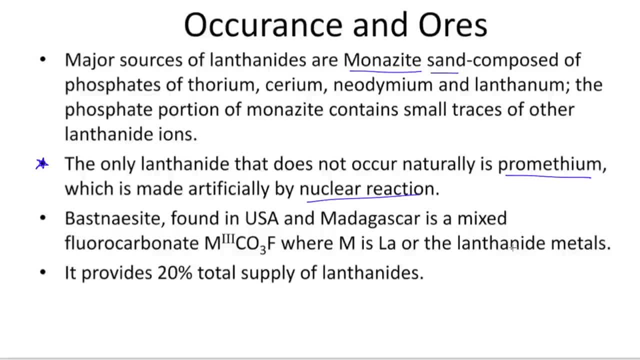 it's a lanthanide over here. right, that means you are excluding the lanthanum over here. uh, here it should be ln. okay, that's a misprint. it should be length ln. okay, so you can just write down ln over here. it provides 20 percent of the total supply of the lanthanide, so this particular ore basnicite is. 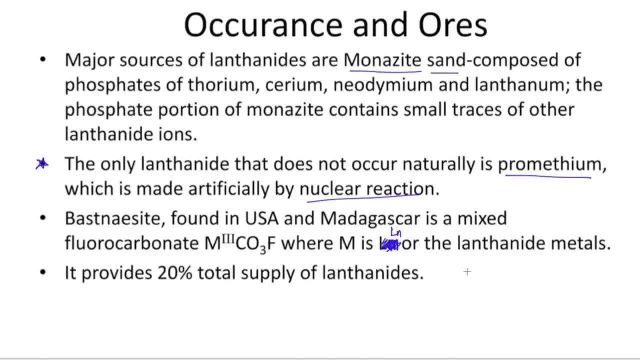 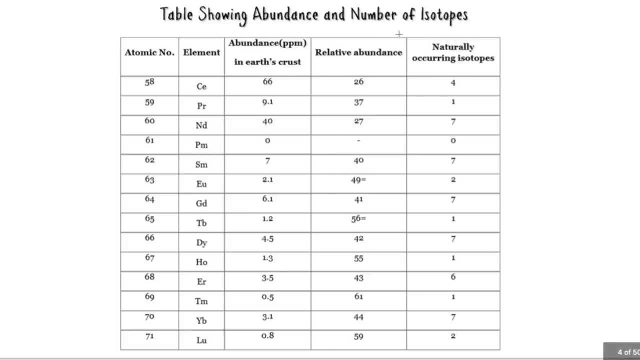 uh, it is of also one of the biggest ore for you- lanthanides. okay, this is about the basics of it. now let's talk about the abundance and the number of isotopes which they have. so these are the different lanthanides which you can see right now. 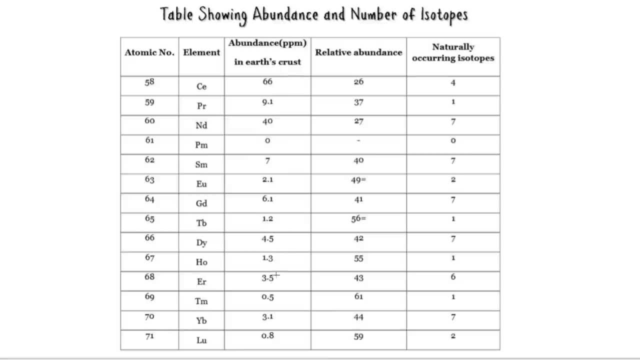 on your screen and these are their abundances, like the different abundance of them on the earth crust, the relative abundance and their naturally occurring isotope uh. at the end of this video, i'll give you a more uh like detailed uh tables, which will show you a lot more information than these. 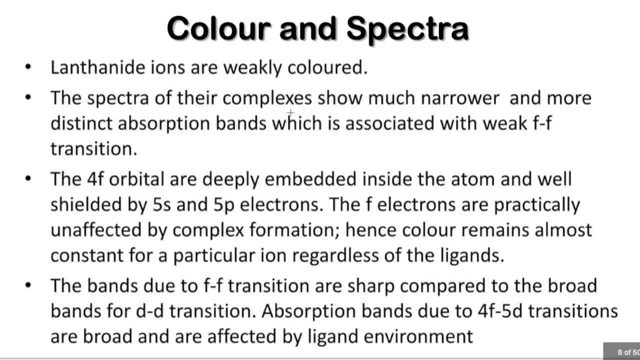 okay, so for now just hold on with me. so the next important thing about lanthanide is their color and spectra. so lanthanides, basically, are weakly colored. same goes for your actinides also. they are also weakly colored. okay. so lanthanides and actinides, both okay. the spectra of their complex show much narrower and more distinct. 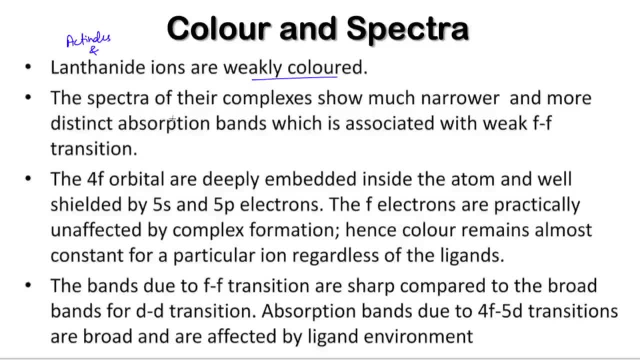 absorption band which is associated with weak ff transition. so these properties are associated with all lanthanides and actinides, both okay, so their spectra has narrower and distinct absorption band, whereas dd transitions are broad and they are not that distinct. okay, and they are associated with ff transition. okay, the 4f orbitals, which are deeply buried or embedded. 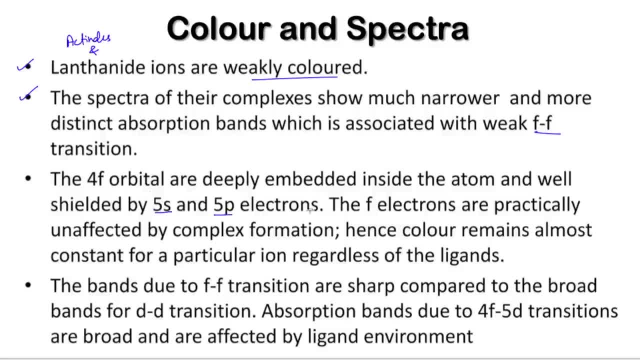 inside the atom and well shielded by 5s and 5p electrons. the f electron are practically unaffected by the complex formation. hence the color remains almost constant for a particular ion, regardless of the ligand. so you need to remember this point: that the color of the complex 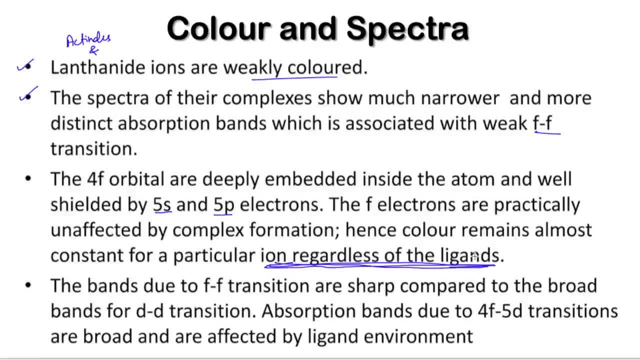 of your f block element, whether it is lanthanide or actinide. in both the cases it does not changes with the ligand. it does not depend upon the ligand environment, it only depends upon uh, the ff transition or the energy difference between the f levels. so the color of the iron, color of the 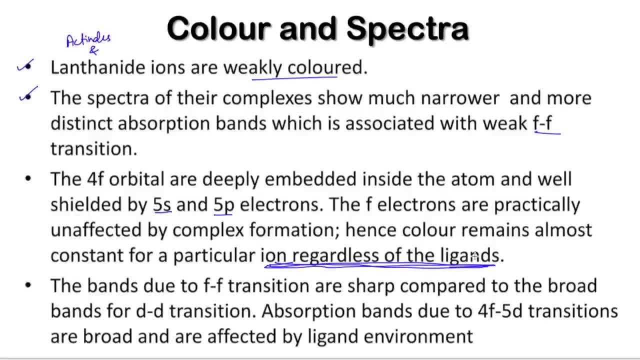 complex. all of them remain quite same because it does not f, like the ligand, does not affect the color of the complex, all right. so this is a very important point. you have to make this, make this sure that you remember left and right. that is why I have chosen. you can see that in dcastド is example here. 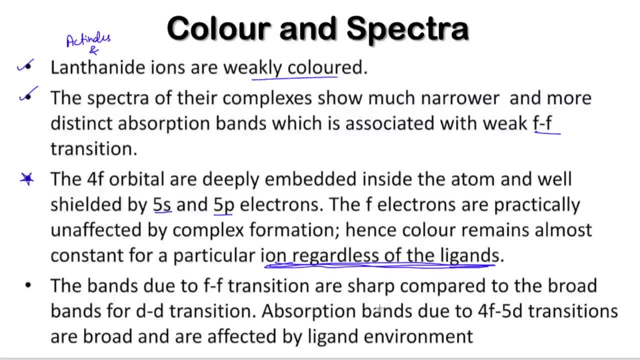 if you can see that, you can see that the application of the complex, so that you might also see- oh yeah, that we'llpg map it this. The next thing says that the band due to FF transition are sharp compared to the broad band of DD transition. So you need to see this point that the FF transitions, which is happening. 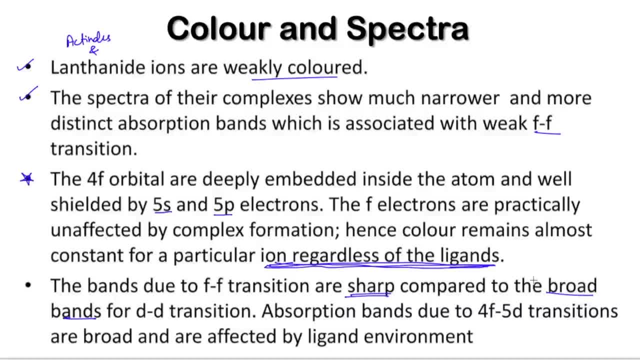 in the F block elements are sharp, whereas DD transitions give you broad bands. Absorption band due to 4F and 5D transitions are also broad and are affected by the ligand environment. So wherever this D transitions come, wherever this D orbitals will come, then the transition will. 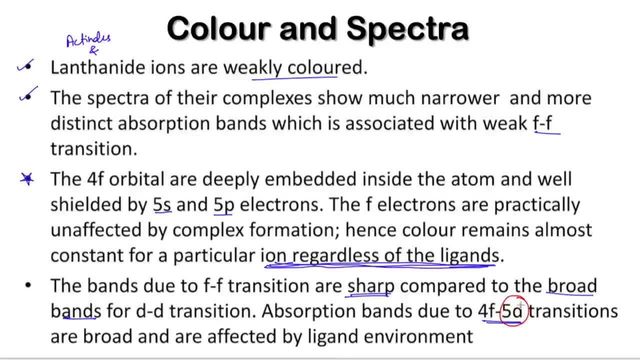 be affected by the ligand environment unless and until you have F orbitals only, like your FF transition. So whether you have 5F- 5F transition or you have 4F- 4F transition, in both the cases they are not going to get in affected by the ligand environment and they are going to be sharp. 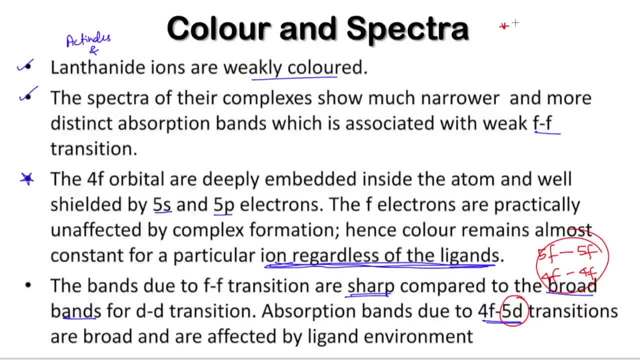 So these are certain points which you can write down: that FF transitions are sharp and they are like, you can say that they are not affected, or unless and until you have F orbitals only like your FF transitions. So whether you have 5F, 5F, 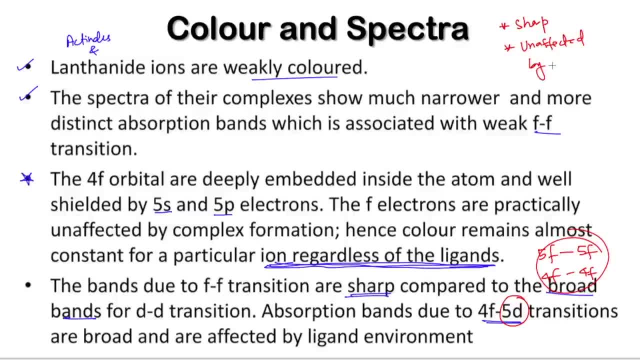 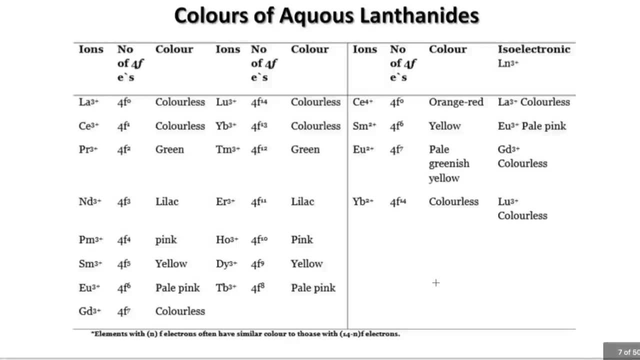 transitions. they are not affected by ligand environment. So these are two very important points regarding your FF transitions happening in your lanthanides or actinides. Let us take the next point, then. So this slide shows you the different colors of the different lanthanide ions. 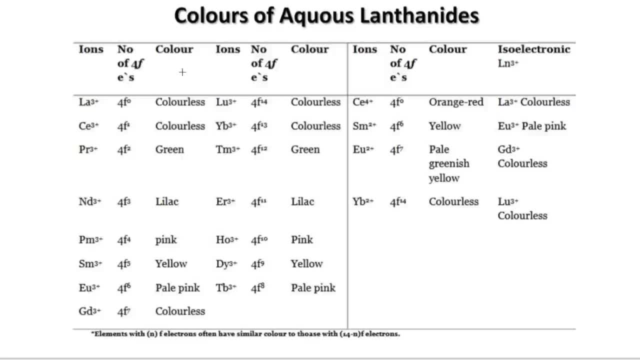 over here. So these are the different tri-positive lanthanide ion. their colors are given to you over here and you can just memorize. So this slide shows you the different colors of the different lanthanide ions and they are given to you over here and you can just memorize. So this slide, wenn-. 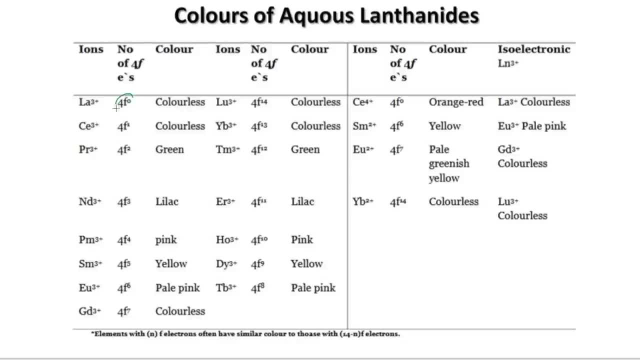 summarize this particular table, you can see one thing, one pattern which you can see over terrified. you can see one thing, one pattern which you can see over terrified is that F0, F14 and F7, all 3 of them are actually colorless. All of them are. 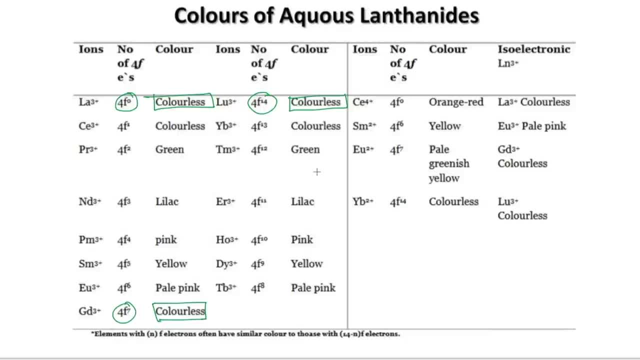 colorless. So you have to see like that. the second important thing which you can look upon this table is that that F1 and F13 have similar colors, Then F2 and F12 has again similar colors. Can F3 and F11 have similar colors? Can F2 and F12 have again similar colors? Can F3 and F11 have again similar colors? 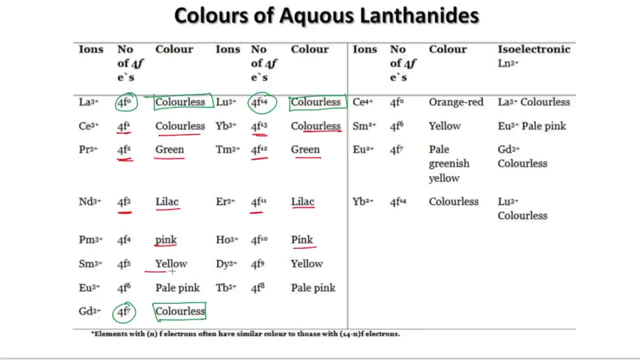 color. so what you can say. you can see it, it is happening in all these things, right in all, like within all the tables. so what you can say? that f n and f 14 minus n, okay, both of them have similar colors, both of them resemble same in color, if the electronic configuration is like that. and the next 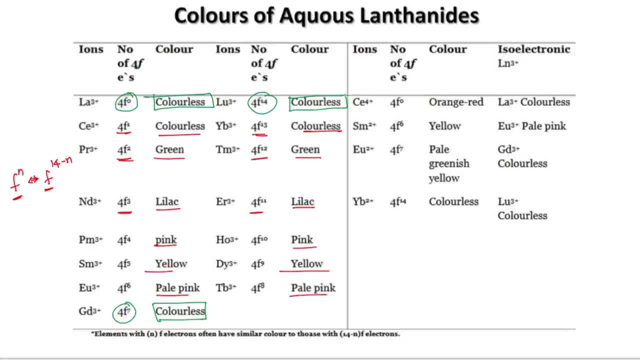 important thing is that their oxidation number should have been same. if you change the oxidation state over here, you can see that your yeah. so if you change the oxidation state, the color changes a little bit like cerium, which stays in plus four oxidation state, then samarium, which stays in plus. 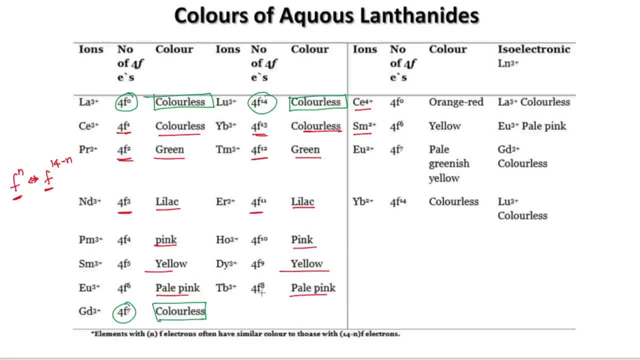 two is yellow in color, and so on. okay, so you just have to memorize these values. okay, so it is iso, electronic, with which? and how does the color like varies. you have to memorize. at least you should memorize this particular table, that's more important, the table which is on the left side. 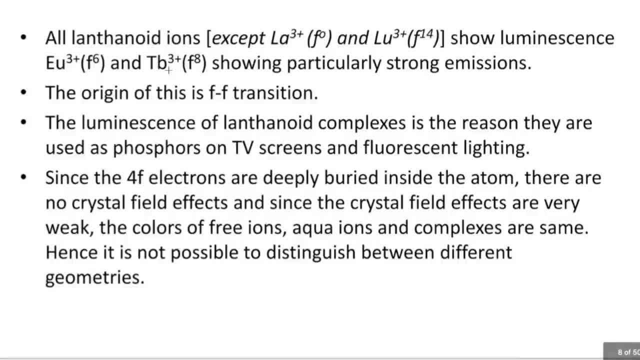 right now. okay, the next important point right now, okay, the next important point right now, okay, the next important point regarding the regarding the uh color and spectra, is that that all the lanthanide ions- okay, except your lanthanum and lutetium, okay, all of them show luminescence, okay, so all the lanthanide. 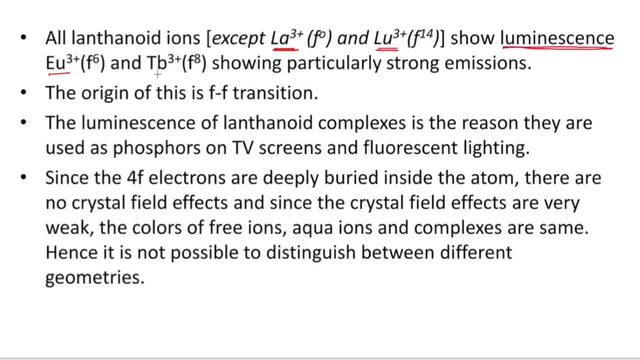 ion shows luminescence, europium and terbium show particularly strong emission. okay, so these are the ones which shows particularly strong emissions, as they are f6 and f8, so they have highest uh ability to do this particular uh like emission spectra, to show the emission spectra. that's why 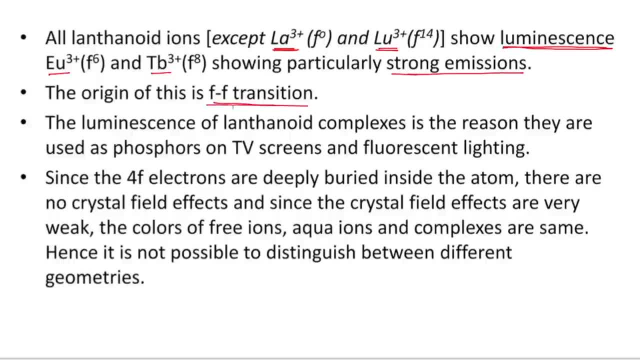 the origin of this luminescence is your ff transitions. okay, the origin of this is your ff transition. the luminescence of lanthanide complex is the reason that they are used as phosphors in the tv screen. we'll talk about that at the later part of this video, where we'll talk 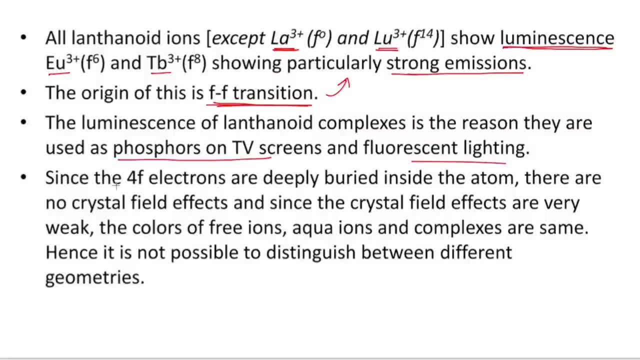 about the uses of them and also using the fluorescent lighting, since 4f electrons. okay, this point is very, very important, so just note this point out and then we'll talk about the effect of ff. in your notebook, okay, in your short notes or wherever you are writing this. that since 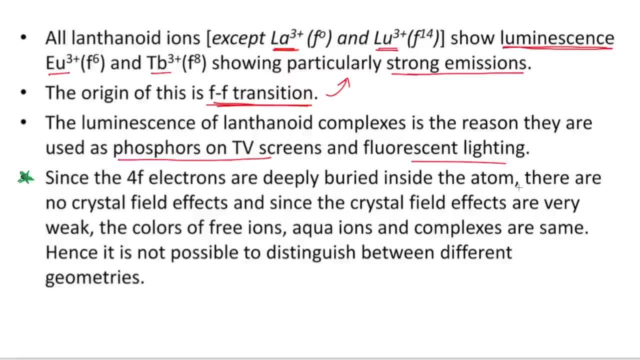 the 4f electrons are deeply buried inside the atom. there are no crystal field effects. okay, there is no crystal field effects which will be there. and since the crystal field effects are very weak, the color of the free ions, aqua ions and the complexes are same. make this thing, make this. 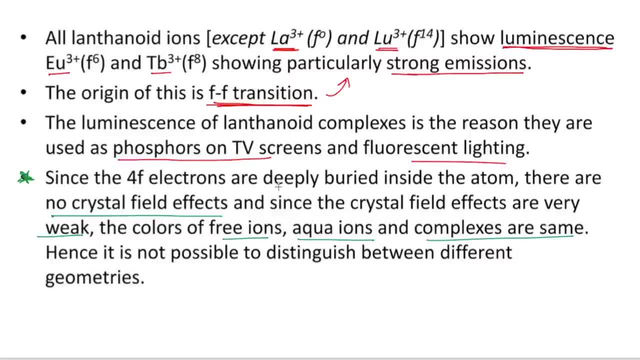 point very clear once again. okay, so since the 4f electrons are deeply buried inside the atom, there is no crystal field effect, there is no crystal field effect. there is no crystal field effect, crystal field effect. and since there is no crystal field effect, they are very weak. 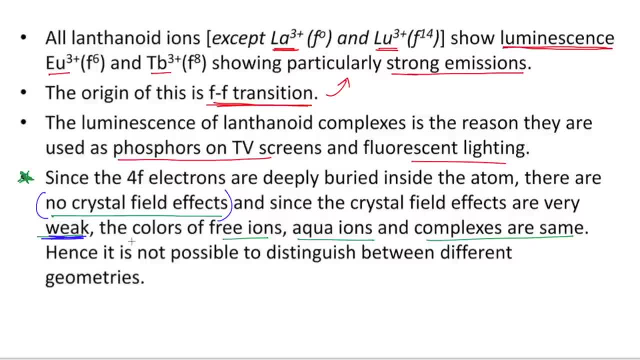 like the crystal field effects are very weak. the color of the free ions, aqua ions and the complexes, basically they all are same Now. hence it is not possible to distinguish them with between them with the help of color. So color of the complex is not going. 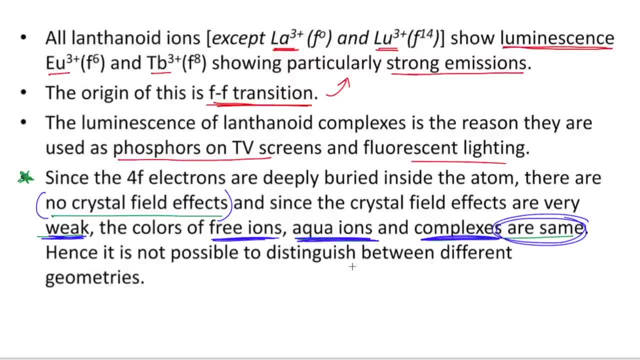 to help you to find out difference in the geometry which you can do in case of d-d transitions or in the case of transition metals. you know that that if you get intense color- probably the complexes of tetrahedral geometry- right, you can do that with the help of your color, but that you cannot do. 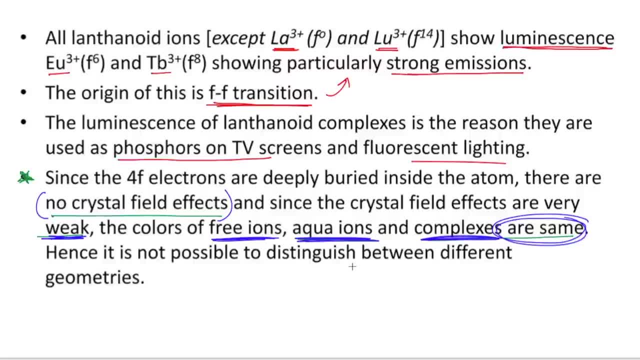 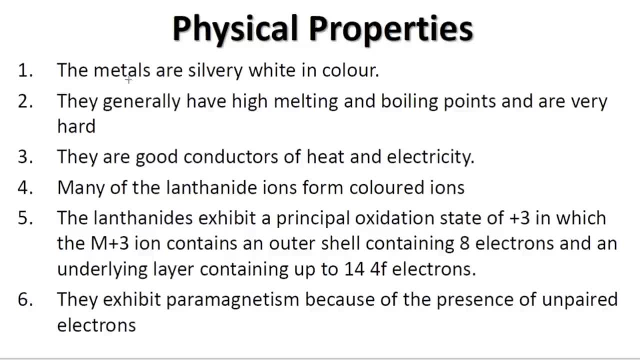 in the case of f-f transitions or in the case of f-block elements. Let us go to the next thing, that is, physical properties of f-block elements. So basically all of them are metal and they have silvery white color. they have generally high melting point and boiling point. both these 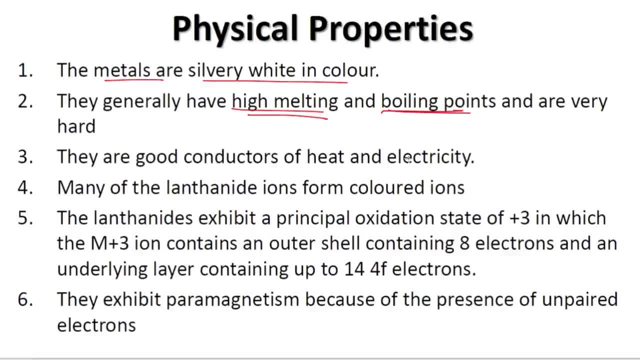 high, like both melting and boiling points are high and they are very hard. this is also important point that they are very hard. They are very good conductors of heat and electricity. many of the lanthanide ion form colored ions. remember this, that the lanthanide ion forms colored ions. but 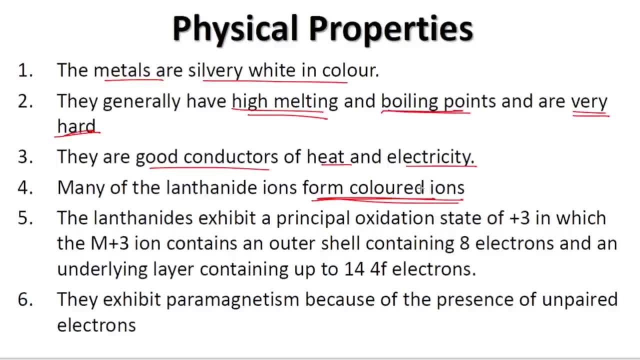 their color is not affected by the ligand field. that also you have to make sure. The lanthanide exhibit a principal oxidation state of plus 3, in which the metal plus 3 ion contains an outer shell containing 8 electrons and an underlying layer containing up to 4, 14, 4 f electrons. So that is. 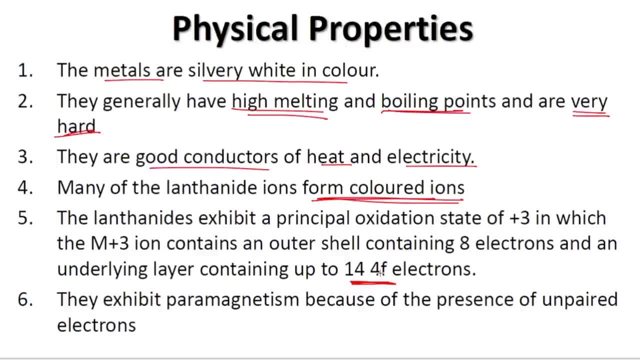 what is given about the lanthanides. So it is start from your shell, like that that you are out like. the 4 f orbital will have electrons from 4 f 1 to 4 f 14. that is what the electronic configuration goes like. Next is that they exhibit paramagnetism because of the presence. 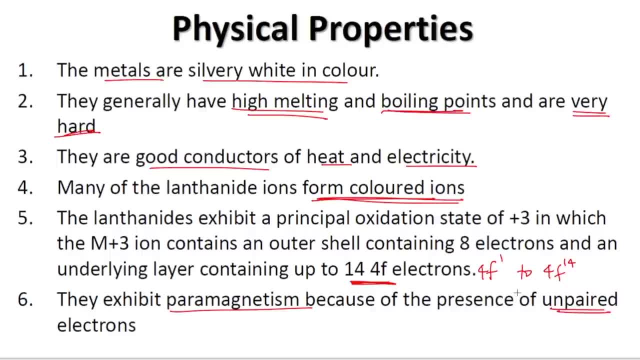 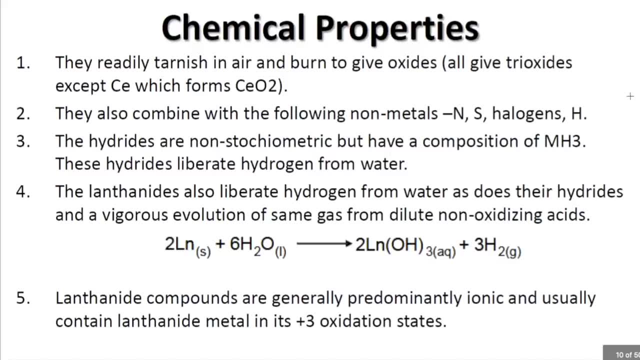 of unpaired electrons, So they have- almost all of them have unpaired electrons, So they have unpaired electrons. So that is why they show paramagnetism in the like in their physical property. Let us move forward to the chemical properties of lanthanides. Now lanthanides. 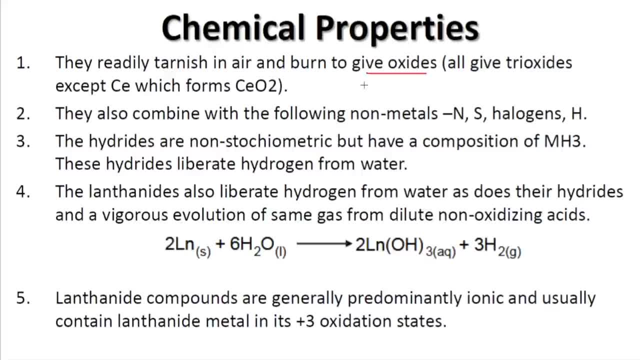 readily tarnish in air and they burn to give oxides. basically all of them, like all the lanthanide gives you trioxides, except your cerium which gives you dioxide. So it is exceptional case or it is like analogous behavior of cerium which you can see over here Now. they also combine with the following: 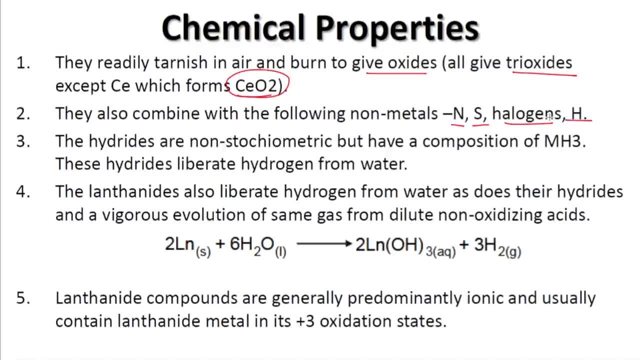 elements like nitrogen, sulfur, halogens and hydride. So these are also some of the elements which combine with your lanthanides. So lanthanide basically reacts with more electronegative elements. that is what you can summarize from this particular point. It needs more electronegative. 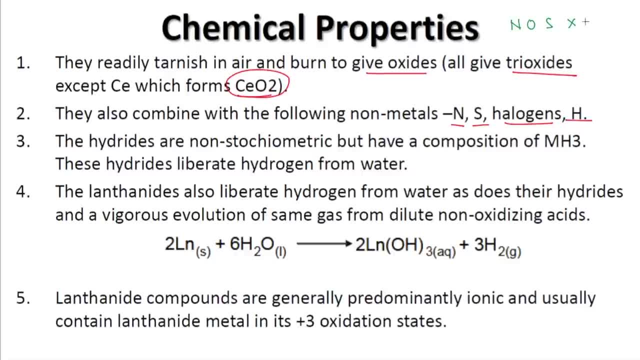 elements like nitrogen oxygen, sulfur, halogens or hydride. The hydride are non-stoichiometric but have a composition of MH3. These hydride liberate hydrogen from water. So that is the chemical reaction. 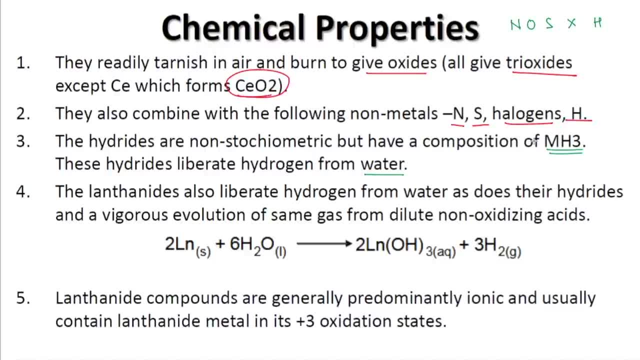 So if you react this hydride with water, hydride will liberate hydrogen gas. Lanthanide also liberate hydrogen when they are reacted with water, when they react with water and they form like hydroxides. So that is what is given to you: A lanthanide reacting with water is going to give. 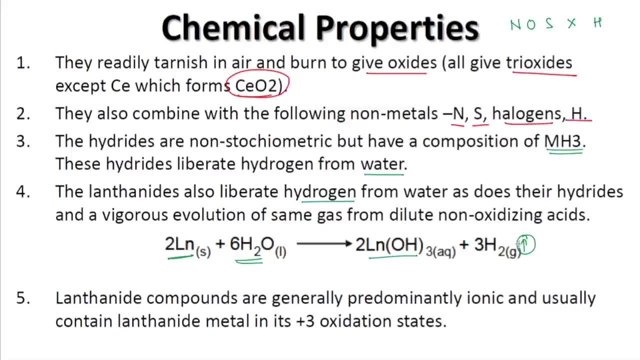 you lanthanide hydroxide. along with that, you will get hydrogen gas, which will be evolved. So that is what is the chemical reaction, which is one of the most important thing. The most important chemical properties of lanthanides, Lanthanide compounds, are generally: 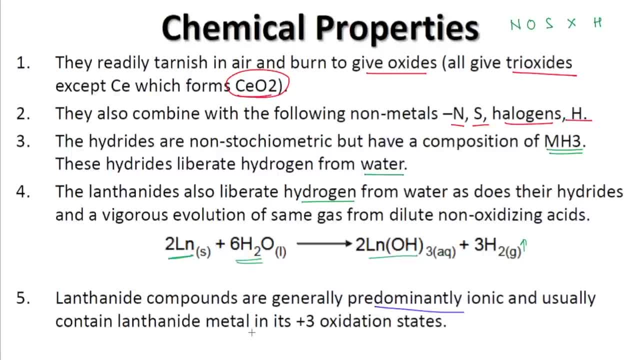 predominantly ionic and usually contain lanthanide metal in plus 3 oxidation state, As I told you, lanthanide element. like they have properties or they have similarities with the group 2 elements. Group 2 elements form ionic bonds, So they also are quite ionic in nature. 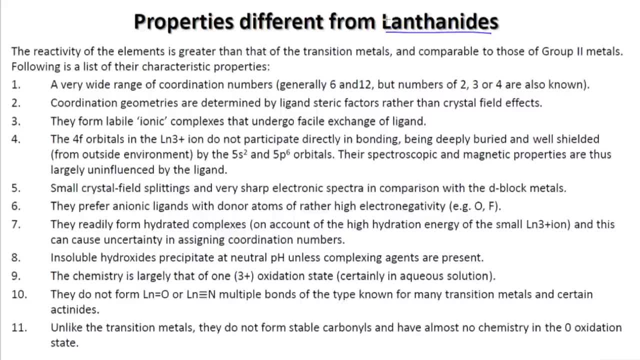 Let's talk about those properties of lanthanides which are different from- sorry, the properties. So let's talk about those which are with the properties, which are different from your d block elements, which are different from your d block elements, or you can say, which are different from your transition. 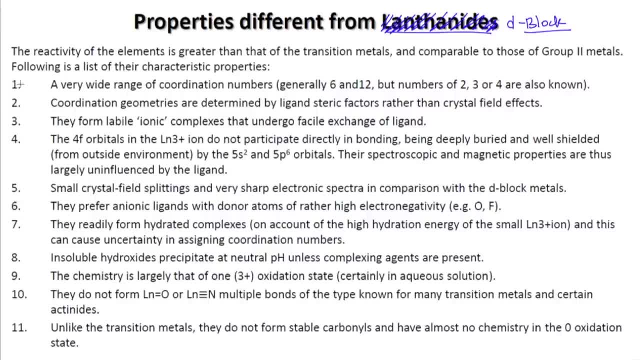 metals. So the first property is that. the first property says that the wide range of coordination number is seen for lanthanides They generally form coordination number of 6, 12, but 2,, 3 and 4 is also known. But in the case of d block element general coordination numbers are 4 or 6.. You don't 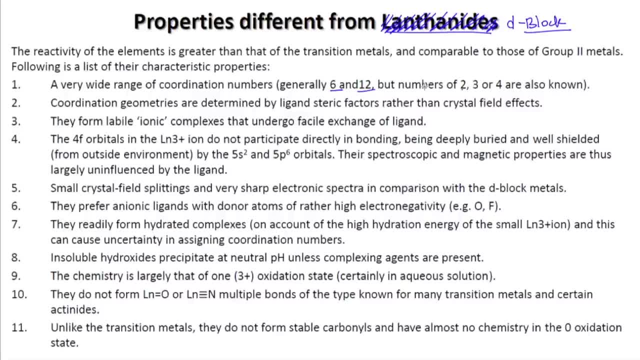 have that much variety of coordination numbers. So you can say that the first property is that the warfare is very reiterate in a closed effect case, image input function in case of d block element In lanthanides you have that. Second point says that the coordination geometry 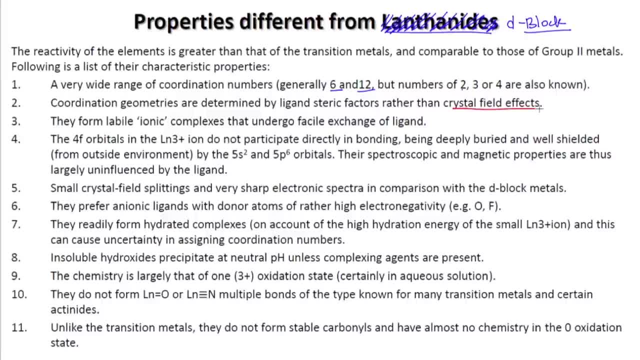 are determined by the ligand stearic factor rather than the crystal field effects. So ligand stearic factors, the stearic hindrance between the two ligand, is going to decide that how many coordination number will be there around a period. lanthanides. 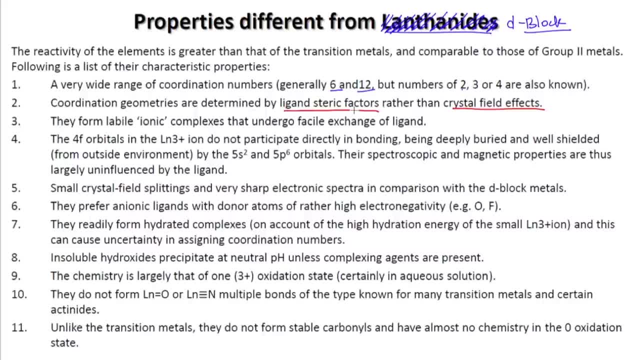 So how many ligands are going to surround a period? lanthanide is going to be decided by the stearic factor of the ligand, not by the like, not by the crystal field effects, that which, the crystal field effects would be determined as the linear flattering. So 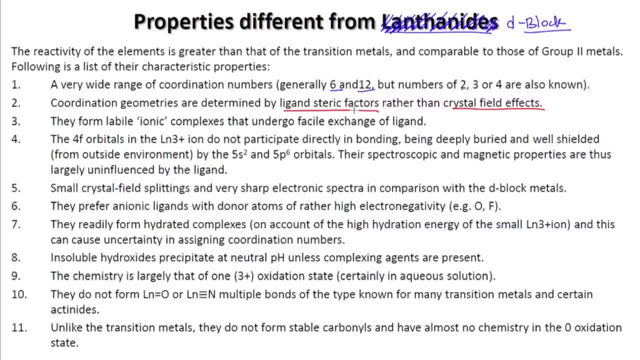 field effect which describes the geometry in the d block elements. that is not going to be used over here. The reason is again the same: because the FF transitions or the F block are involved in the in these and there is no like they are deeply buried inside, So they do not get affected by the. 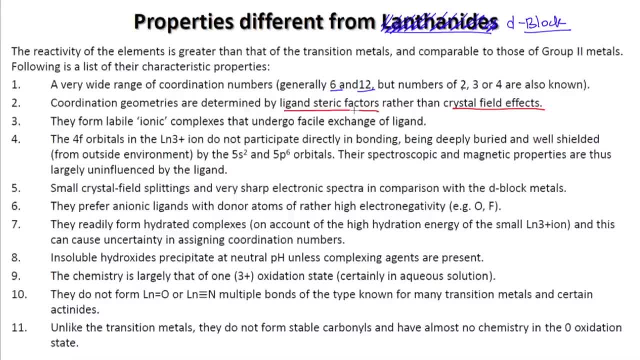 ligand field. that is why So no crystal field effect, but yes, steric effect is there. So a bulky ligand will be less like. let us say, if I have bulky ligands So they will form less coordination number complex, a smaller ligand or a or a less bulkier ligand is going to form more. 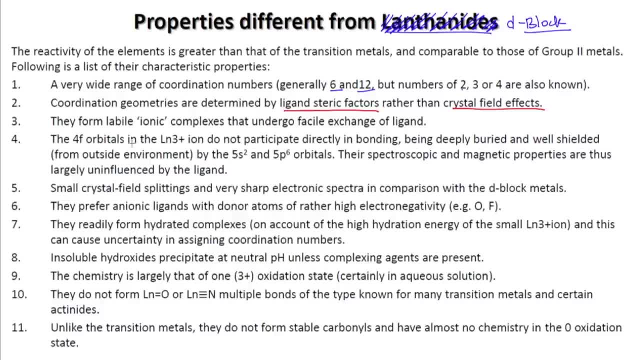 coordination complex with the lanthanide. that is what it means. The next thing is that they form labile complexes. you have to be very careful with these terms. So they form labile complexes and they undergo facile ligand exchange. 4F orbital in the lanthanide plus ion do not participate. 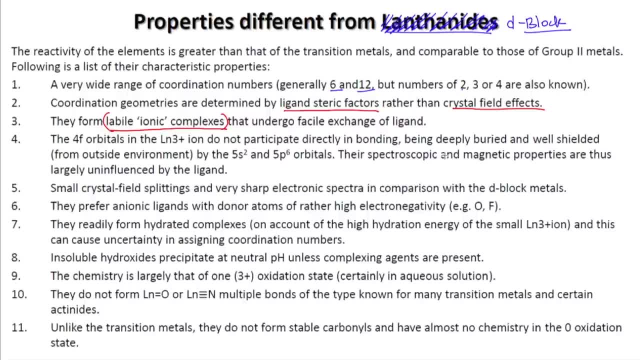 directly in the bonding, being directly, being deeply buried inside and well shielded by the 5s and 5p orbitals They respect. the spectroscopic and magnetic properties are largely uninfluenced by the ligand. We have discussed this point quite a bit of time, So you might have understood this by now. So their spectroscopic 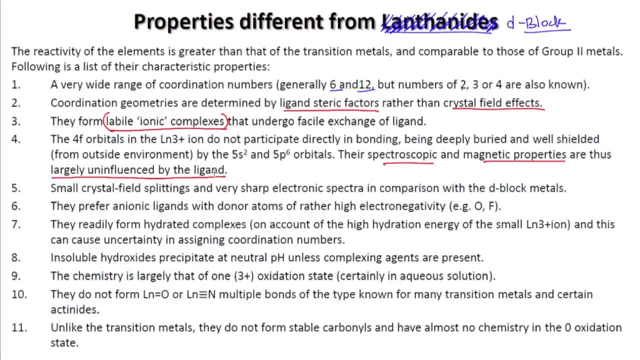 properties means their color and spectra, and their magnetic property is also not affected by the ligand. Small crystal field splittings and very sharp electronic spectra is observed in comparison with the D block elements. So in F block element you see that you have small crystal field splitting. the region is again same, which we have discussed in the previous point. 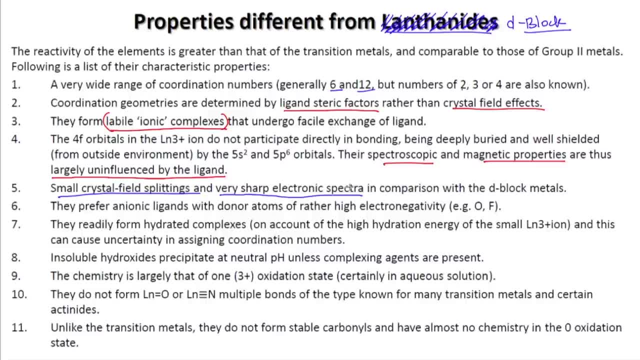 and they have very sharp electronic spectra, whereas in the D block elements we have high crystal field splitting and broad electronic spectra. So that is the major difference between both of them. The next thing is that they prefer ionic ligand with donor atom rather than high 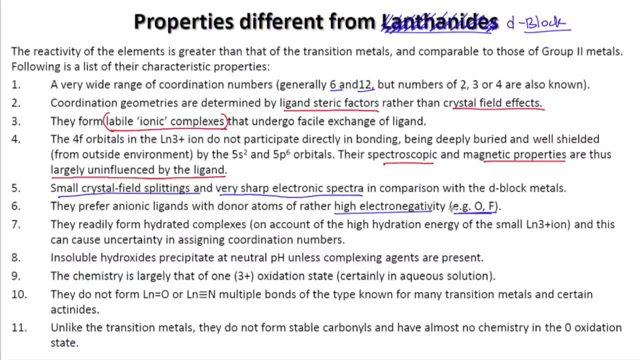 electronegativity, So they react with those donor atom which have high electronegativity, whereas D block elements react with those elements also, those ligands also which do not have high electronegativity, like your carbonyl ligand is there, and these are the ligands which do not have much electronegativity, yet they 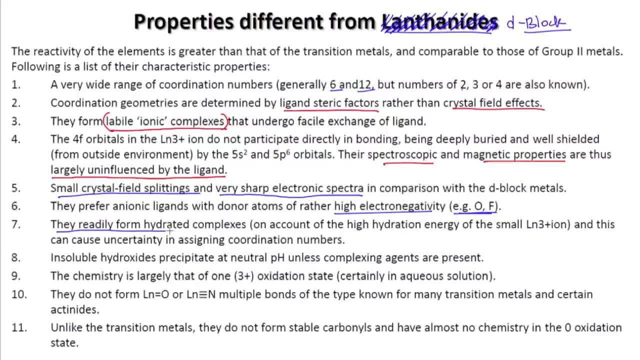 react with the D block elements, They readily form hydrated complex. we have seen that and on the account of high hydration energy of lanthanides and this can cause uncertainty in assigning the coordination number. So the coordination number is basically a part of your steric factor. The insoluble hydroxide precipitate at neutral pH unless complexing. 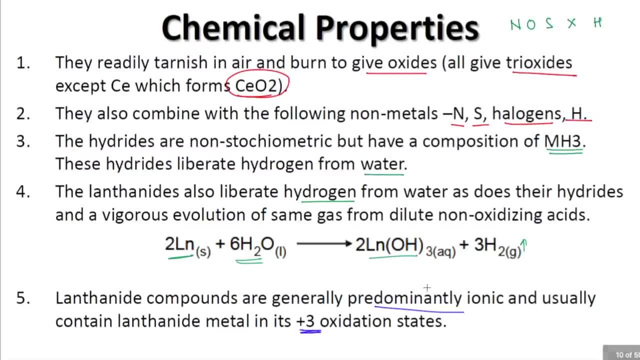 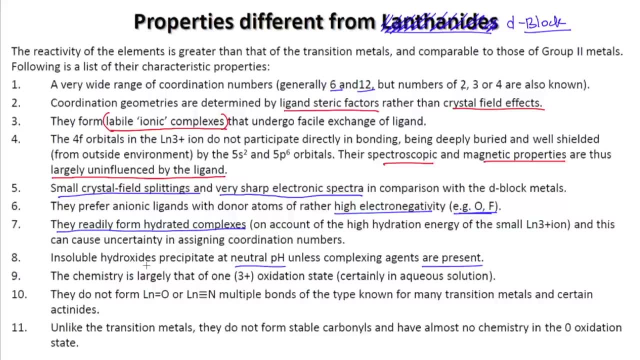 agents are present. Understand this thing. you have seen in the previous chemical properties that hydroxides were formed. Now these hydroxides are insoluble and they generally precipitate at the neutral pH, unless and until you put some complexing agent. Now these complexing agents have a. 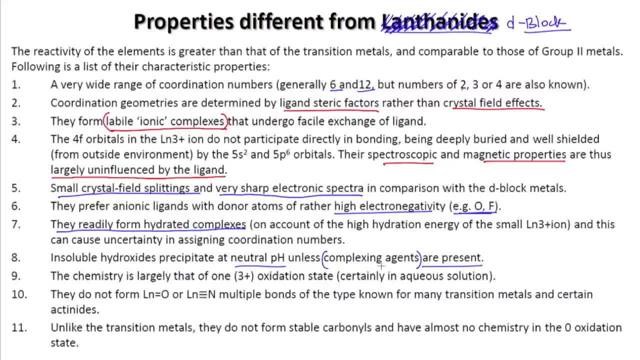 property to form complex between lanthanide hydroxide and the solvent and do not allow them to precipitate and let them like, let them stay in the solution. So that is what is the property or that is what is the use of the complexing agent. The chemistry is: 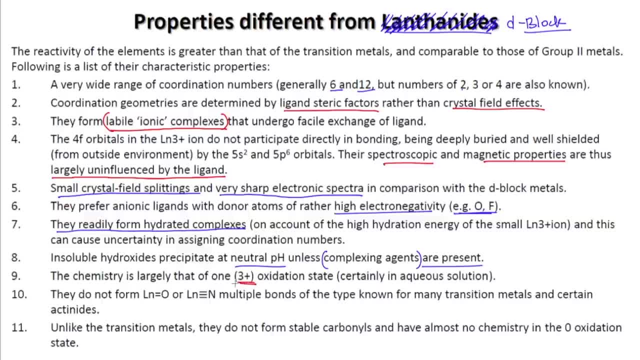 largely that of plus 3 oxidation state for the lanthanides, whereas in the D block elements the chemistry is for the variable oxidation state. you have seen even plus 7 oxidation state in case of manganese, two plus one oxidation state in case of like titanium and copper. 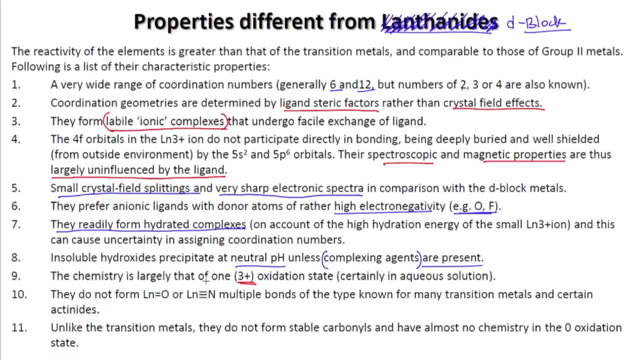 So there are variable oxidation states in the D block elements, but F block elements generally have plus 3 oxidation states. They do not form double bond with oxygen or triple bond with nitrogen. So you can see that then these nucleic acids, in this case, are oxidized. 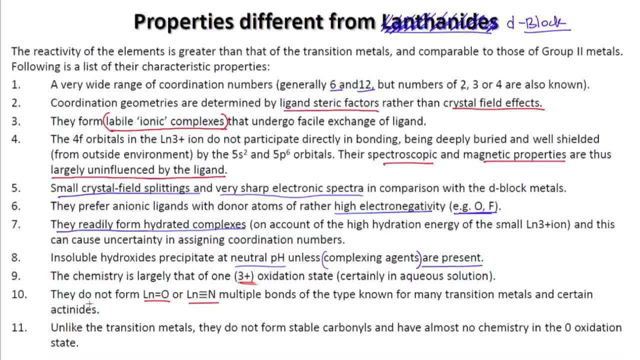 Therefore, nucleic acid is essentially oxidized by ferric acid nitrate, so they are oxidized. So these are oxidized by ferric acid nitrate. so they are oxidized by ferric acid nitrate. So of the type known for many transition metal and certain actinides, so certain actinides also form. 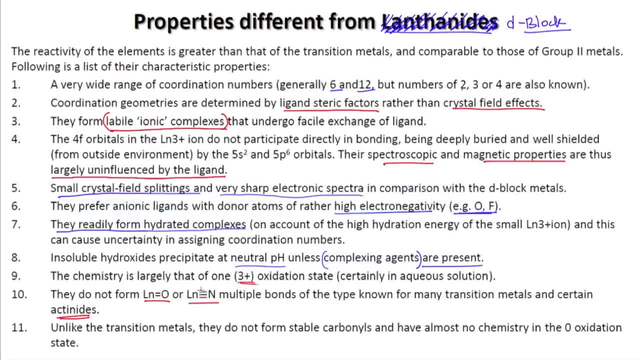 this triple and double bonds. but lanthanide do not do that. okay, unlike the transition metals, they do not form stable carbonyls and have almost no chemistry in the zero oxidation state. so they do not have any chemical reaction or any chemically known substance in the zero oxidation state. so do 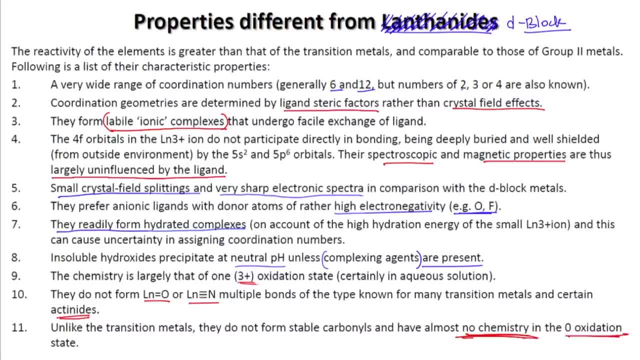 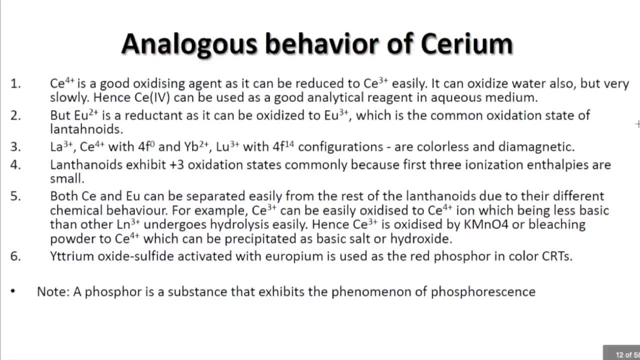 so they do not have carbonyls of them or lanthanide carbonyls are very rarely known, or they are actually not known up till yet. now let's talk about the analogous behavior of cerium now. so cerium is one of the element which has very analogous behavior. the first of them is that cerium 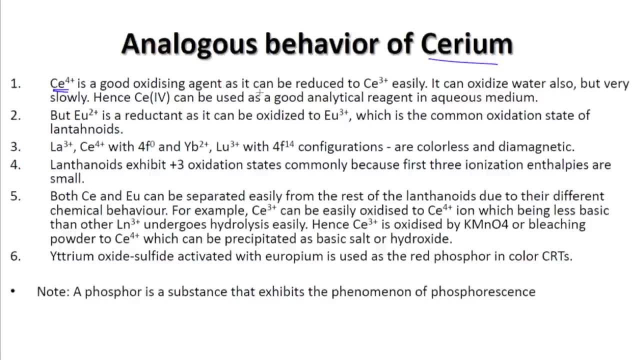 in plus four oxidation state is a good oxidizing agent as it can be reduced to cerium plus three easily and it can oxidize water also, but very slowly, okay. hence cerium plus four can be used as a good analytical reagent in the aqueous medium. you have seen, there are many organic reagents. 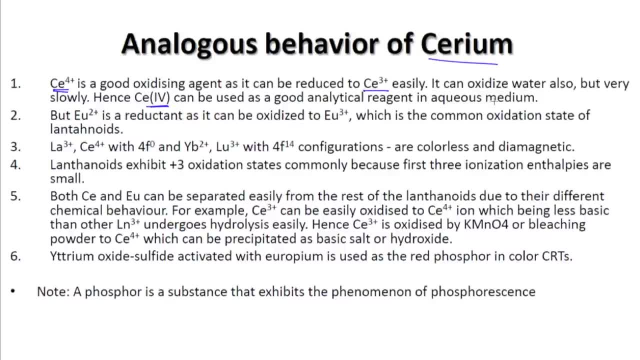 which have cerium in plus four oxidation state. i would like to know from you guys how many like did you guys remember any of the organic reagent or any of the reagent which is having cerium in plus four oxidation state? if you know that, do let me know in the comment sections below. 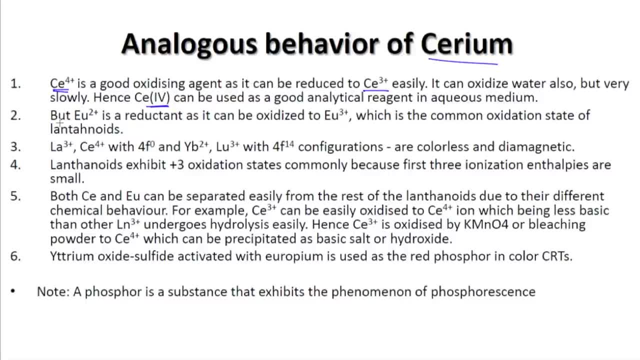 the next thing is that the next point is that europium plus two is a reductant and it can be oxidized to europium plus two, which is a common oxidizing state of the lanthanide. so basically, these are the two different oxidation states which we have seen so generally. lanthanides gives you plus three. 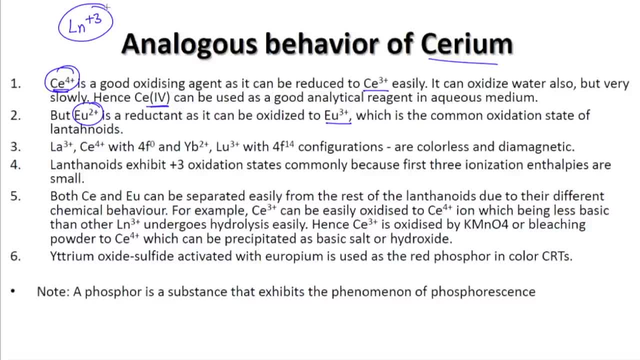 oxidation state. apart from this plus three oxidation state, there are various other oxidation states also known only for these two elements. like for cerium, we have plus four oxidation state. europium gives you plus two oxidation state rest. other elements are not known to give variable oxidation state. okay, so lanthanum plus three, cerium plus four with four f. 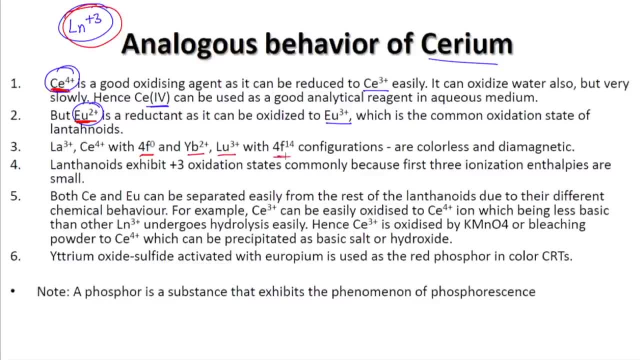 and yttribium plus two lutetium plus three with four f14 configuration. they are colorless and they are diamagnetic. i told you that most of the elements, or most of the lanthanides, are paramagnetic, except these four. okay, one, two, three and four. these four are diamagnetic and colorless. lanthanide exhibit. 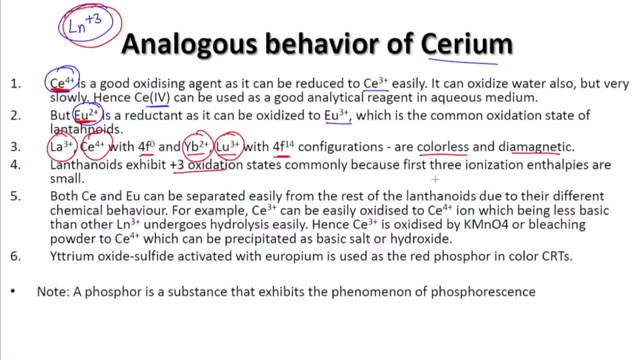 plus three oxidation state commonly because first three ionization enthalpies are very small. both cerium and europium can be separated easily from the rest of the oxidizing state, so this is also known for the lantnides, due to their different chemical behavior. okay, for example, cerium plus three. 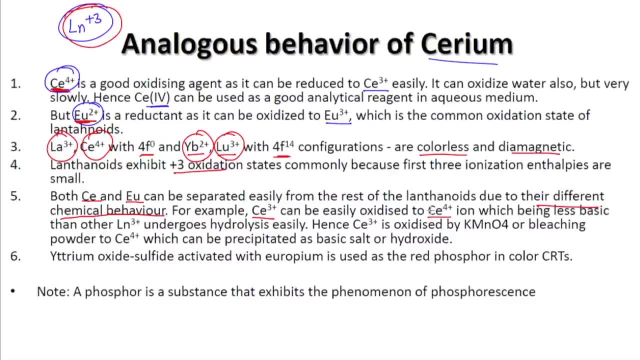 can be easily oxidized to cerium plus four, which is less basic than the other lanthanide ion, and thus that's why it can be hydrolyzed easily and it can be separated out. okay, so hence, cerium plus three is oxidized by caminophore, or bleaching powder, to cerium plus four, which can be precipitated. 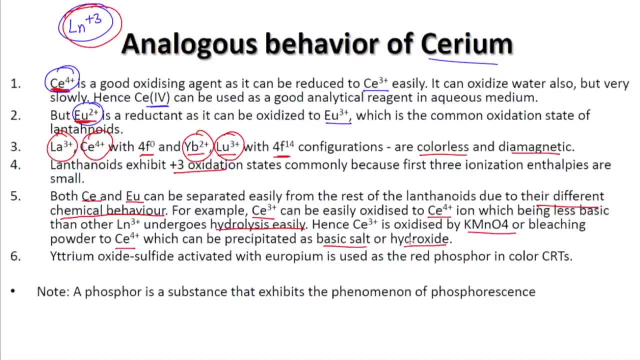 as a basic salt or as a hydroxide. so from the rest of the salt, like from the rest of the mixture of the lanthanide ion, you can easily separate out your cerium plus four. In the same way it is easy to separate out European plus 2, because their oxidation states. 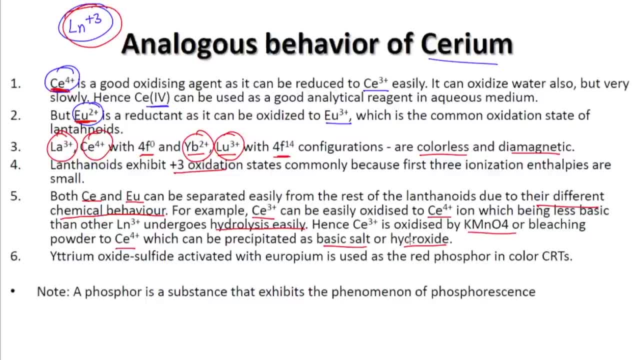 are different Rest of them, which are having in plus 3 oxidation state. they can be separated by a method called as ion exchange method. ion exchange method. Let us talk about the next point, which says that the atribium oxide sulfide activated with European is used as a red phosphor. 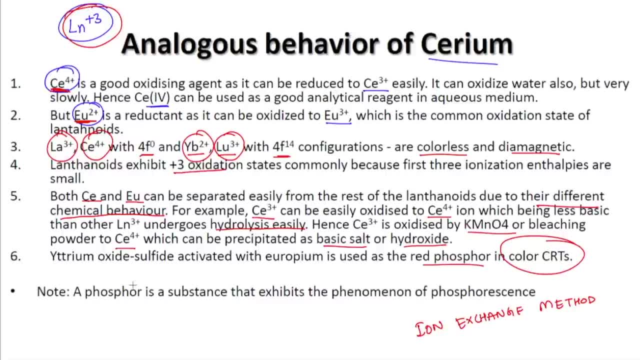 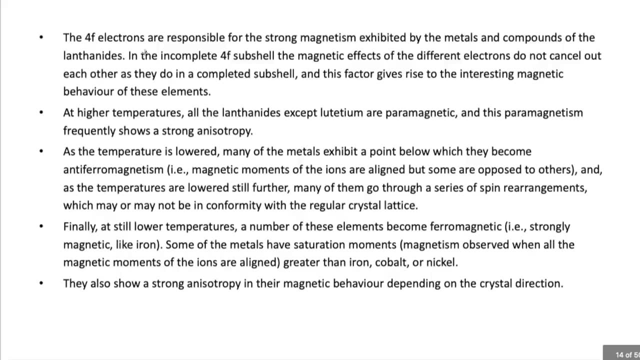 in the color CRTs. So what is a phosphor? Phosphor, basically, is a substance that exhibit a phenomenon of phosphorescence. So when the light falls on this phosphor, it shines, It gives you a certain color out of that. Let us talk about the magnetic properties now. So the 4F electrons. 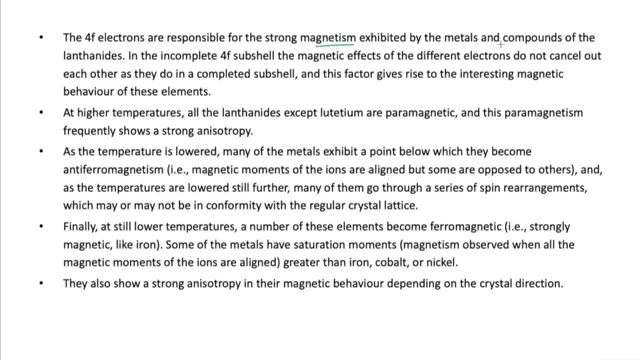 are responsible for the strong magnetism which is exhibited by the metals and the compound of the lanthanides which we know In the incomplete 4F subshell. the magnetic effect of the different electron do not cancel out each other and they do. 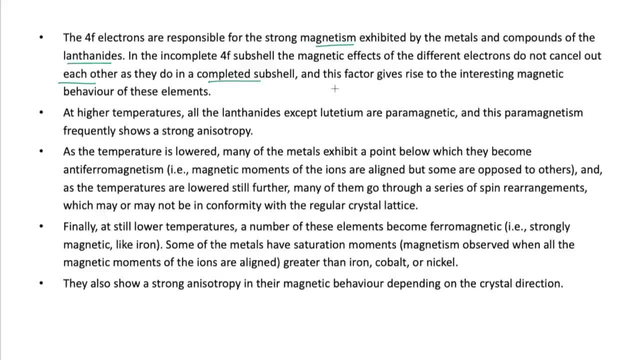 As they do in the completed subshell, and this factor give rise to interesting magnetic behavior of these elements. So there is a very interesting magnetic behavior which you are going to get to know. So at higher temperature all the lanthanide except lutetium are paramagnetic. So all the 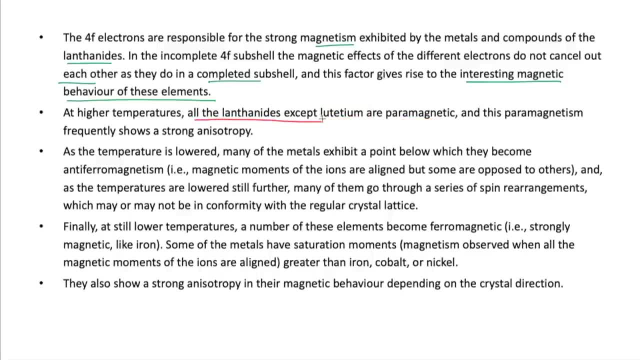 lanthanide, except lutetium, is paramagnetic at higher temperature. So make this thing very careful, Note it down somewhere. And this paramagnetism frequently shows a strong anisotropy. Now the next thing is that, as the temperature is lowered, many of the metal exhibit a point below which they become. 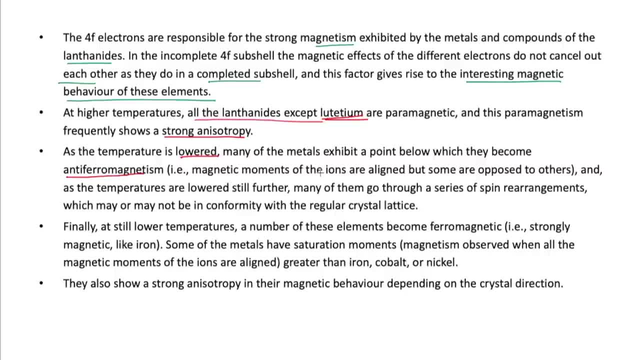 anti-ferromagnetism, That is, magnetic moment of the ion are aligned, but some are opposed to the other. So you know what anti-ferromagnetism means. And as the temperature is lowered still further, many of them go through a series of 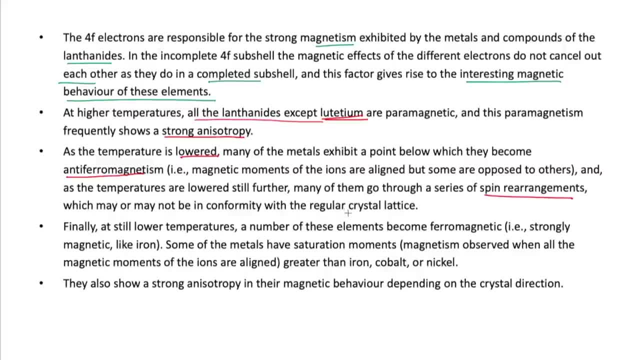 spin rearrangement which may or may not be in conformity with the regular crystal lattice. Finally, at the still lower temperature, a number of elements become ferromagnetic And some of the metal have saturation moments greater than the iron, cobalt or nickel. So that is what it is At high temperature. 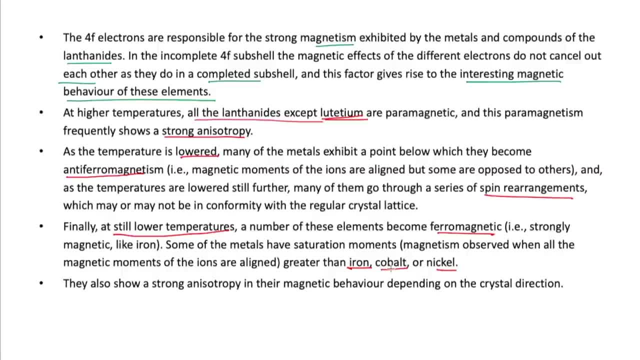 they are paramagnetic. You lower down temperature, they become anti-ferro. If you lower down the temperature more they become ferromagnetic. They also show a strong anisotropy in their magnetic behavior, depending upon the crystal direction. So that is also one of the property. 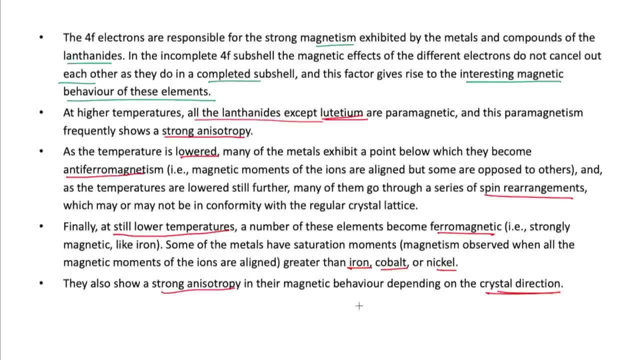 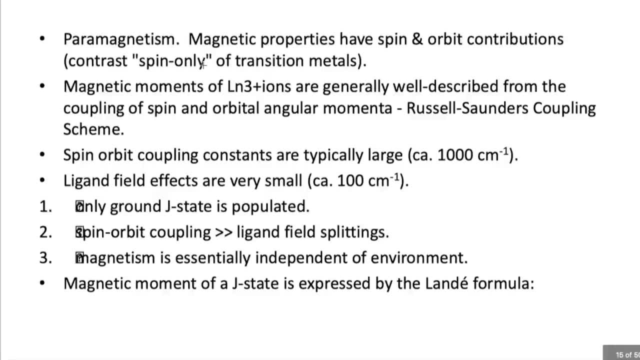 that they exhibit different like value of the magnetic moment if calculated or if that is measured along the different directions. Magnetism is one of the properties, magnetic properties- having a spin orbital contribution. Basically this point, you need to remember that they have spin orbital contribution. Magnetic moment of lanthanide ions are generally well 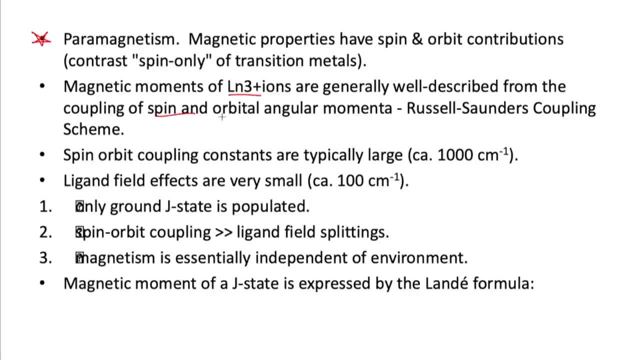 described from the coupling of spin and orbital angular momenta. That is called as your Russell-Saunders coupling. Russell-Saunders coupling scheme and spin orbital coupling constant are typically large. in this case, That is, around 1000 centimeter inverse. So in that, in this way, what happens? What are the consequences of these? 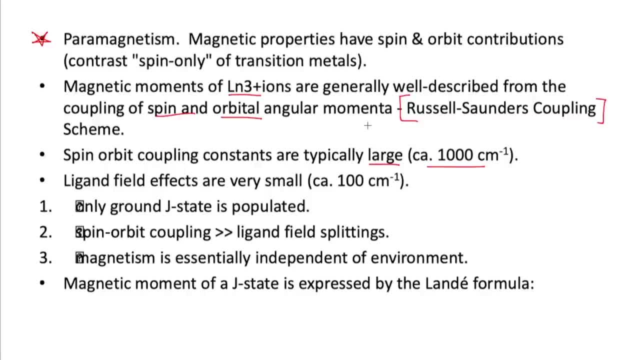 things because of high spin orbital, like spin orbital coupling. What happens? That only the ground J state is populated. The ground J state remains populated. You know the J states right. So the ground state remains. You have studied this in quantum mechanics and you have studied. 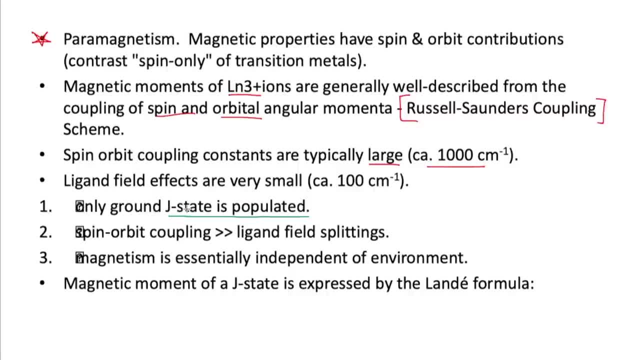 in molecular spectroscopy regarding the J max level and all. So that is what it is mentioned over it, that the ground J state remains populated. So that is what it is mentioned over it, that the ground J state remains populated. Spin orbital coupling is quite large. Then the ligand fill. 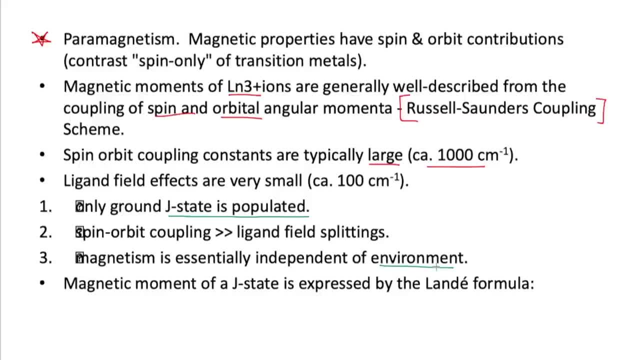 splitting, and that is why magnetism is essentially independent of the environment. These are the three factors which describes the and like exceptional behavior of the magnetism of these lanthanide elements. So that is why their magnetism or their magnetic moment is not calculated by spin only. 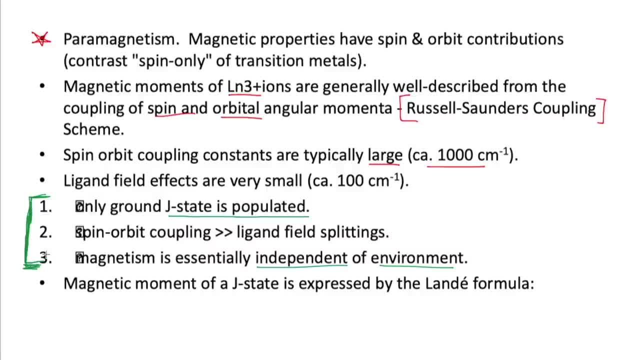 magnetic moment or the formula which we were using for the d block elements. Those formula are not enough to calculate the magnetic moment, So that is why they are not calculated by spin, only magnetic moment. So that is why they are not calculated by spin, only magnetic moment. So that is why they are not calculated by spin, only magnetic moment. So that is why. 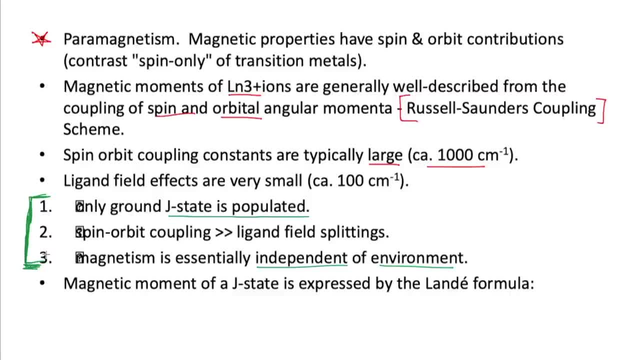 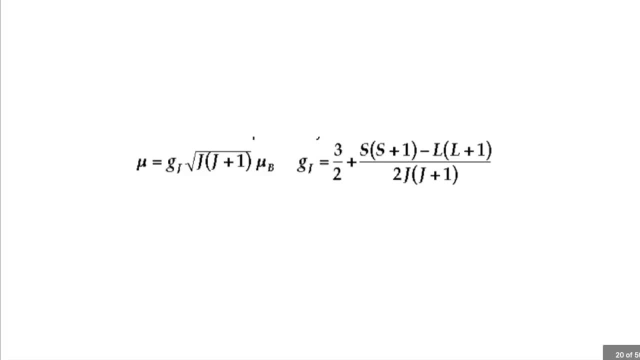 you need certain different formula for that So magnetic moment of these, like J states are expressed in the form of Lande's formula, and I will show you what that formula is actually. So the formula is given by this, It is given by mu is. 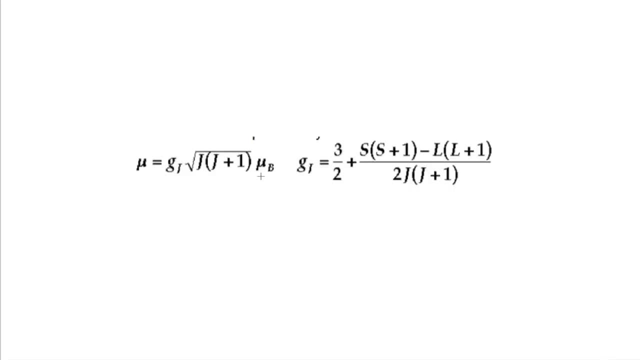 equals to G under root J? J plus 1, and where your G is given by 3 by 2 plus S? S plus 1 minus L? L plus 1, divided by S? S plus 1 minus L? L plus 1 divided by 2jj plus 1. you know what s what l and j are right. all right, so let's talk about certain terms, which. 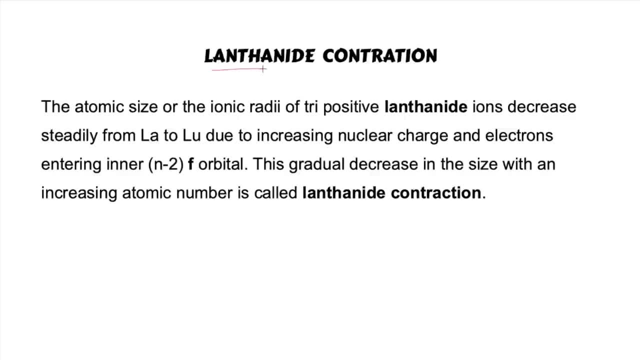 are associated with your f block elements and one of them is your lanthanide contraction. now you know that what lanthanide contraction actually is. it's kind of a revision for that right. so what happens? that the atomic size of the ionic radii of the tri positive lanthanide ions they decreases. 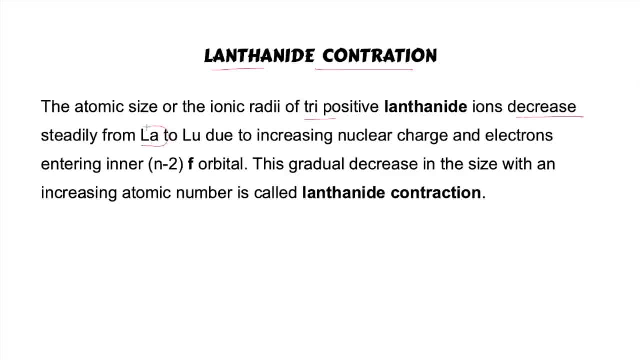 with, like they decreases steadily from lanthanum to lutetium. so when you move from lanthanum to lutetium, the size or the, the atomic size or the ionic radii basically decreases of all the tri positive lanthanum ions or lanthanide ions. so that's because of the increase in the nuclear. 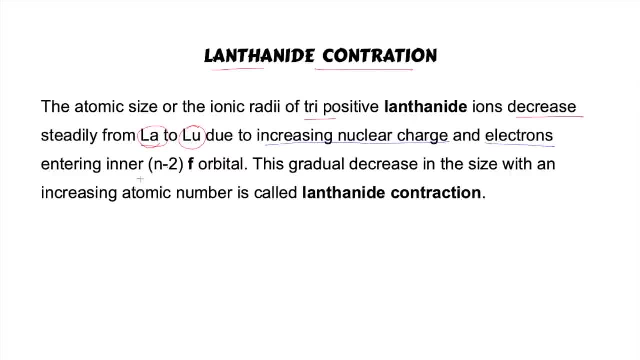 charge and the electron, because the electron enters in the inner n minus 2 f orbital. that's why the nuclear charge increases and because of that there is a decrease in the ionic radii. now this gradual decrease in the size with the increase in the atomic number is called as your lanthanide contraction. okay, so that's what is lanthanide? 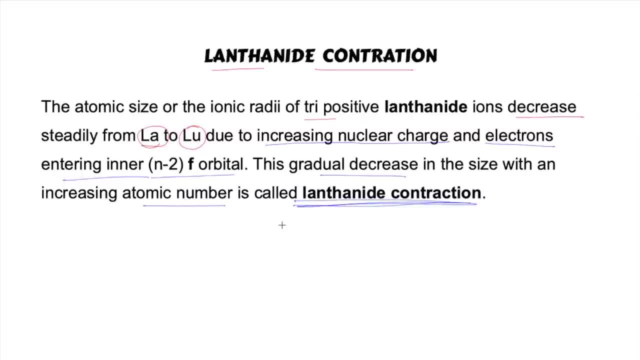 contraction. now it happens in lanthanides, but it happens in lanthanide and actinides both. basically it's called as lanthanide contraction, but similar effect is seen in actinides as well. so although it is called so, but its effect or the application of that is observed in the d block elements and 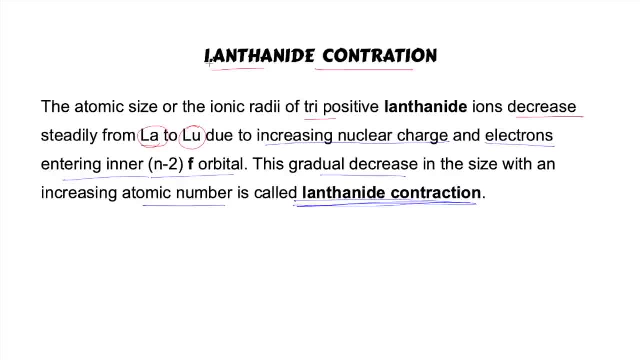 that's why the size of the lanthanum and the hofnium is not that different. okay, they have quite similar sizes, although there are 14 elements between them. these are certain very basic things which you need to know, apart from lanthanide contraction. 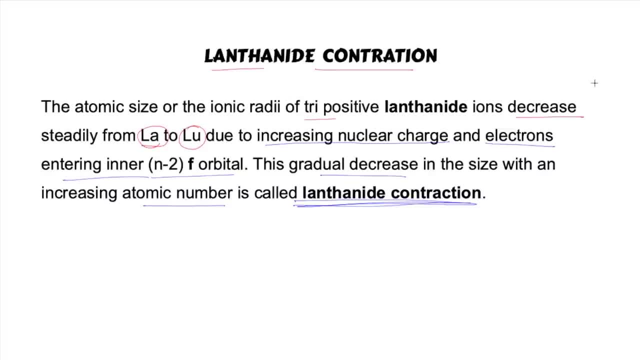 one more concept, actually, which you should study and which you should read, is your ion exchange method. okay, I didn't included it in this particular video because it will make the video too long. I didn't want it because it's a complete different method and you will find a. 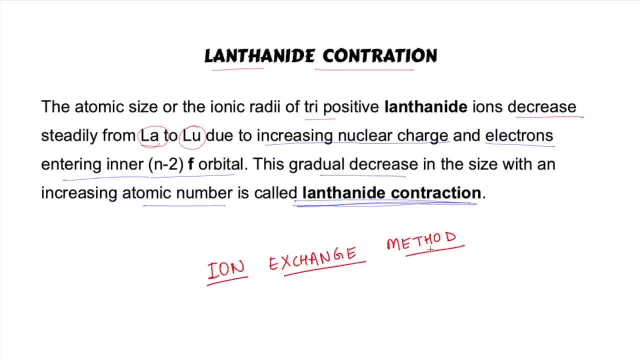 lot of text regarding this and I would recommend it you to read it from books. okay, which like it. you don't have to remember the complete step, you just have to know the certain points, that which element will come first during the ion exchange method. so I'll just give you that that. 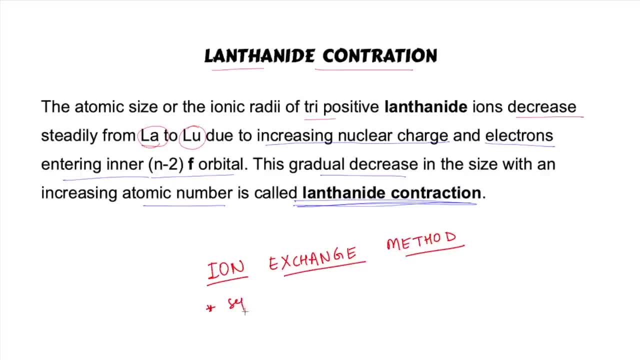 the ion exchange method in. during the ion exchange method, the separation- okay, the separation of smallest, smallest ion takes place first. okay, takes place first. so who will come out of the ion exchange column? if I have the ion exchange column, I will have the ion exchange column, I will. 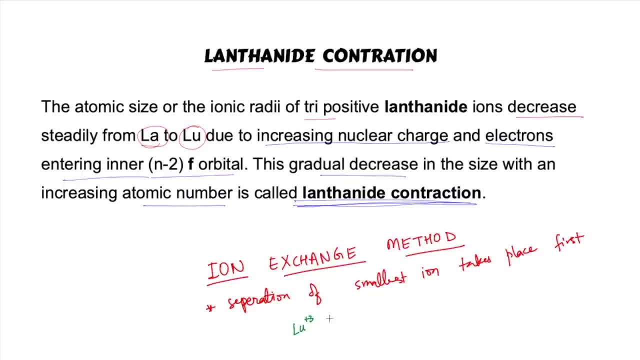 have. so the order goes like this: lutetium plus 3 will come out first, okay, then your yttribium plus 3, and so on. okay. so, based upon the size, this will come first and then this yttribium and all, and that's because the lutetium is smallest in size among all the lanthanides, right? so this is the. 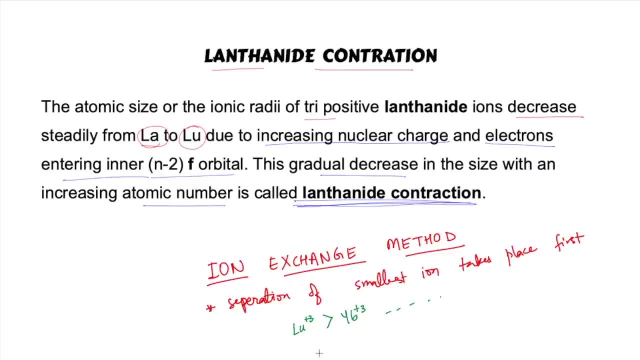 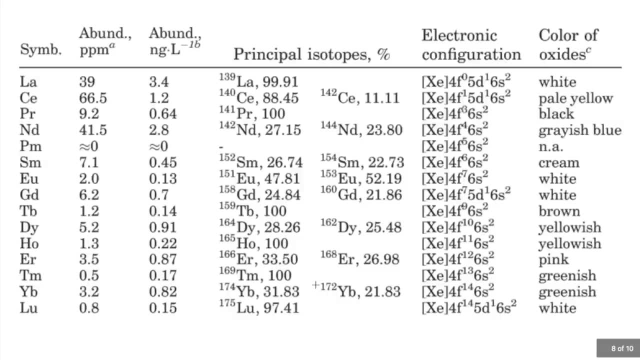 one of the point which you need to know. if you want to study ion exchange method, you can completely study that, but at least this is something which you should know about that. the next thing which I will give you is matrix, because it is or you don't know. now you are gonna remember, is thetag which is: 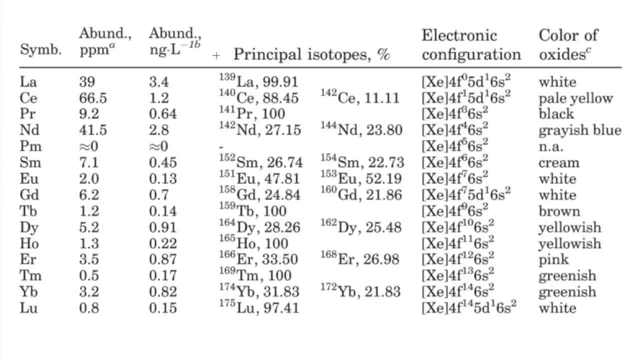 equal to thefinitude of the tone. right, and we are going to know about so number in this workshop when we are gonna do the analysis or we are going to go through dose bra function. you remember that there is assort of molecules with with very high対 non willing if the double n is greater than b, because 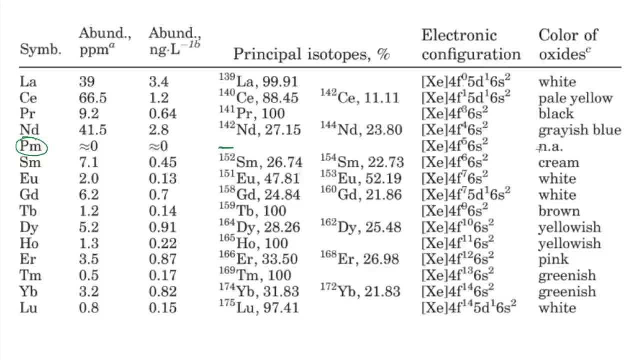 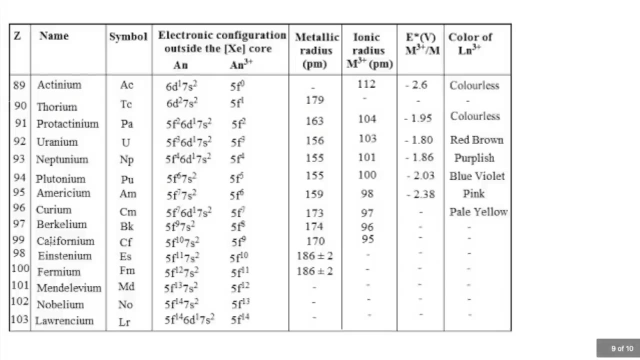 because i told you it is not found on the earth crust, right, and it does not have any any color as well, so you need to remember that. rest of them, you have to just, uh, like, you just have to memorize them, right, uh, apart from them, there is one more table regarding your actinides. now, all the actinides. 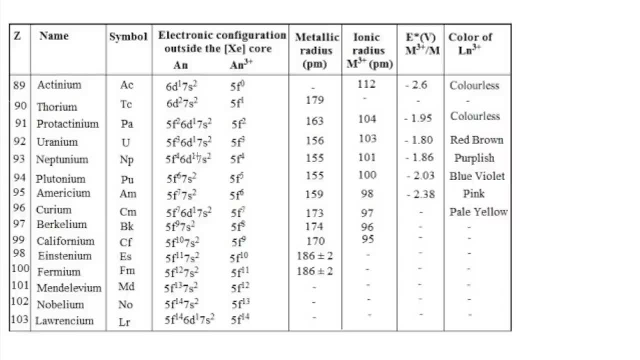 are given over here. their symbols are given to you. these are the different electronic configurations of this plus three ion. actinium are denoted just like lanthanums are denoted by ln. actinides are denoted by an. now, remember i have not discussed much about actinides because most of the properties 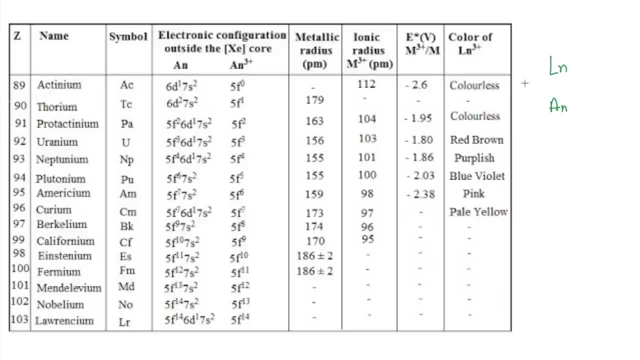 are similar for both of them. uh, the only differences are mentioned over here. you can see these are the like: instead of 4f they will be 5f elements. uh, their metallic radii. you can see that the metallic radii is decreasing and basically these are metallic radii. so ionic radii basically is. 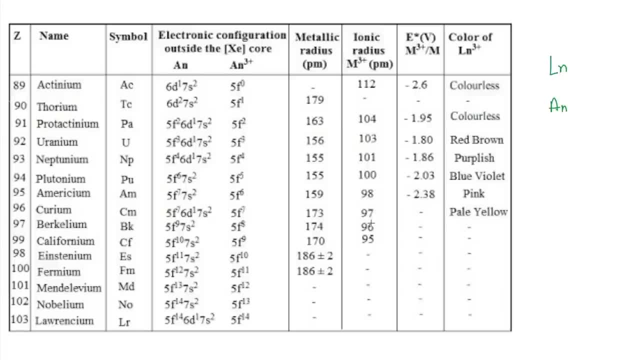 decreasing because of the lanthanide contraction, which you will see here as well. these are the different reduction potential of them. you can see that the ionic radii is decreasing because of the lanthanum contraction which you and these are the different colors of them, the one which are given dash. that means they do not. 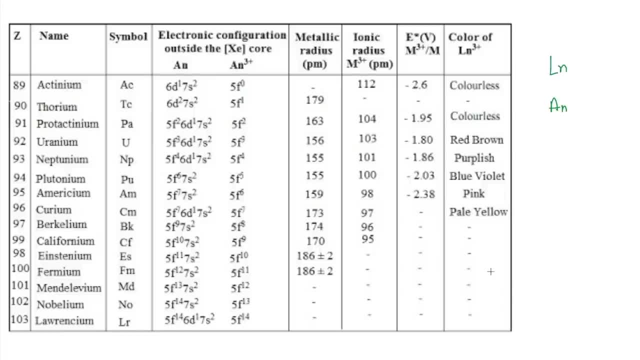 exist. they have been prepared, um like by artificial means, so that's why they do not have any color they are. they are produced by the nuclear reactions. so these are certain things which are there. apart from them, what you have to do is you have to study the theory of your like. some of the 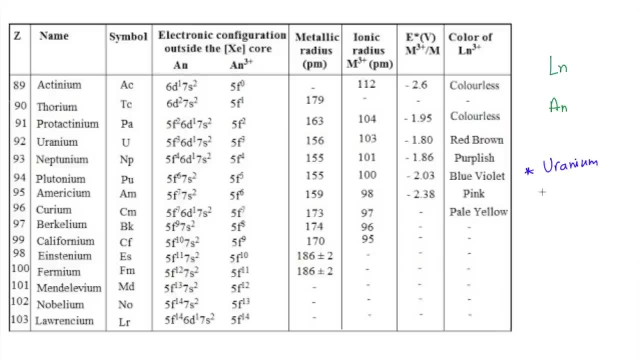 properties of your uranium chemistry. okay, uranium chemistry is something which you have to study now, remember you need. uranium chemistry will also get linked with your nuclear chemistry, so you have to cover all of them and rest of the thing is completed in this particular video. it's a kind of 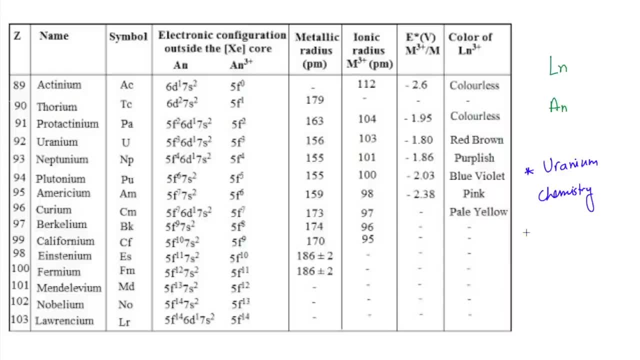 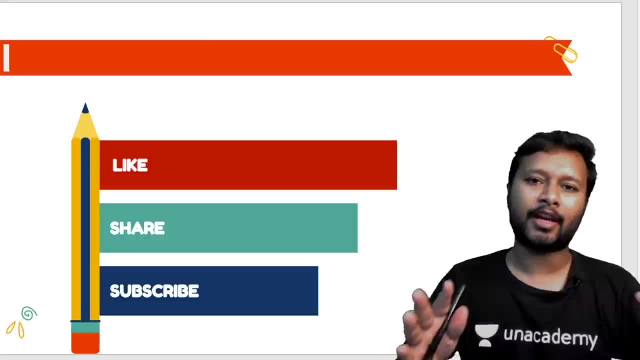 revision, one which would have helped you to revise all the concepts at a particular place. all right, guys, that's all for this particular video. i hope that whatever i have given you in this video, whatever text or whatever topic or whatever notes i have shared with you regarding the f block elements. 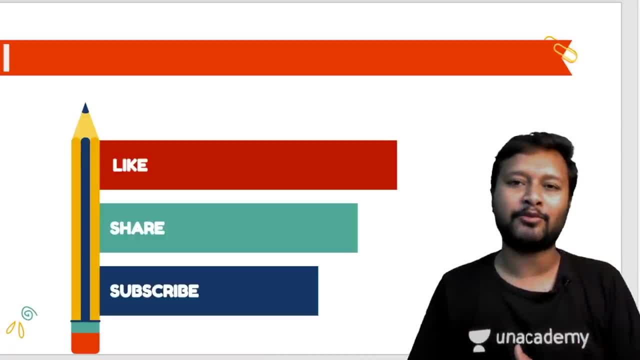 was helpful to you and i hope that you have found this video helpful and if you have any questions. you guys have got to know quite a few new things and if you like this video, please let me know in the comment sections below, and i would like to share the pdf of these slides as well. so if you, 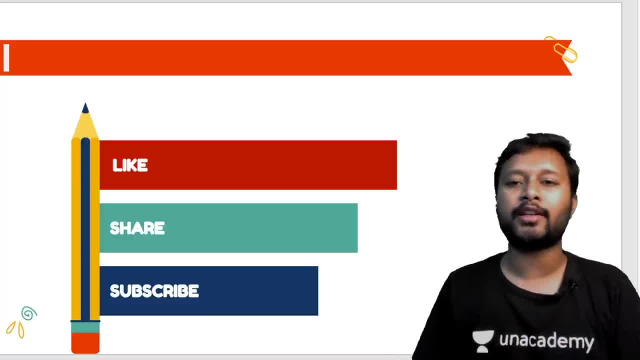 want. so the pdf of this particular content is available in the description of this video, so do check that out as well, and that's all from my side, guys. thank you so much for watching. if you are new to this channel, do subscribe to the channel. if you like this video, give it a like. 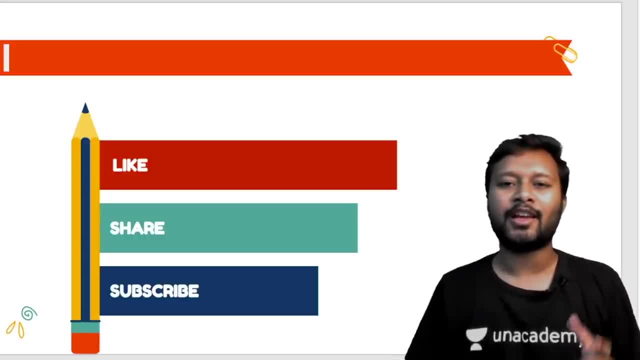 and share it with your friends. so thank you so much for watching and have a great day. bye. 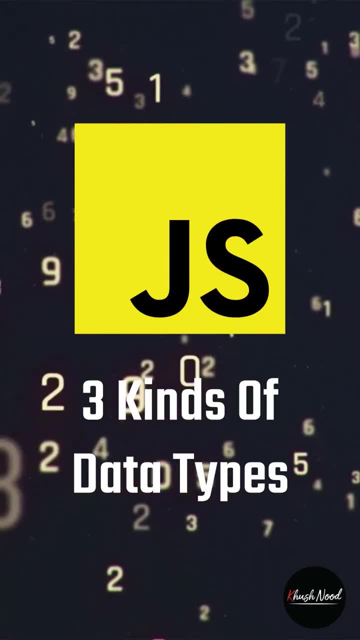 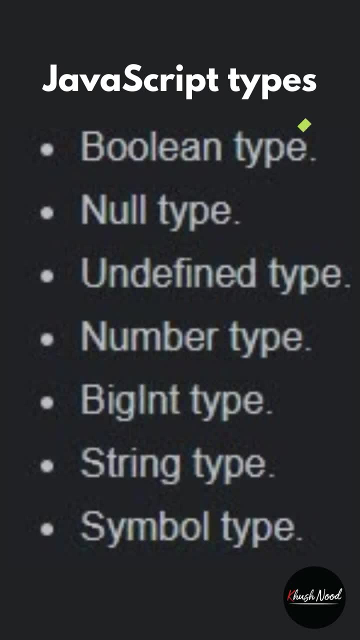 hey guys, in this video i will let you know three kinds of data types in javascript. by the way, javascript has a seven kinds of data types, but in this video we will covering three types of data types: boolean, string and numbers. string is a sequence of letters which is used. 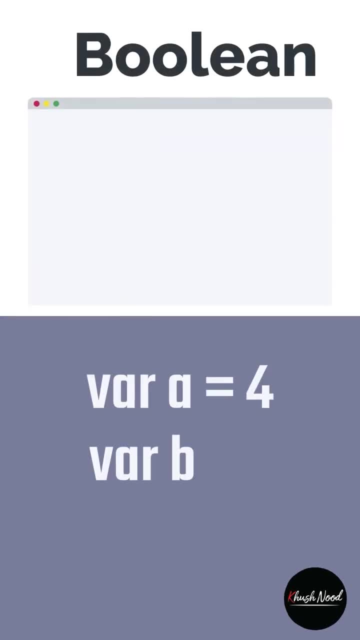 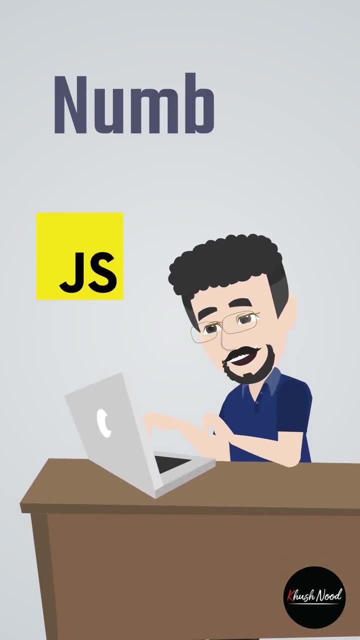 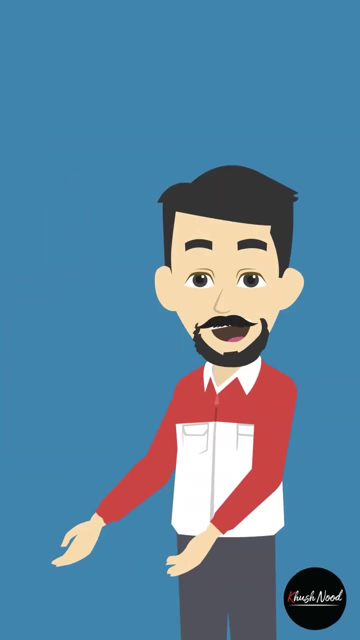 to show any message in the browser. and the other side is boolean. boolean help us to define any statement, whether it's true or false. and the last one is numbers: number help us to put decimal and integers into number. so these are three javascript data types. i hope you.